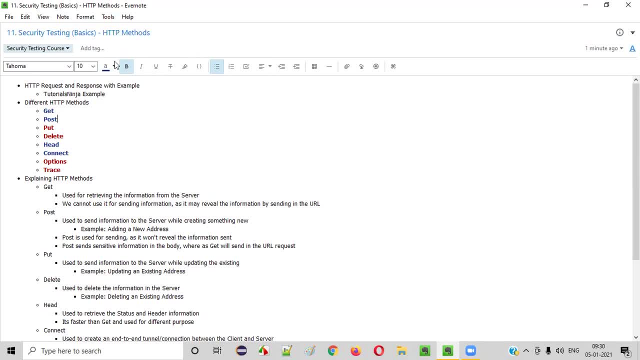 Fine, so let's get started, guys. So before I list down all the HTTP methods for you and explain what exactly these methods are, first I have to cover one basic topic, guys, a concept I need to explain. Fine, let's go through this concept, after that I'll explain. 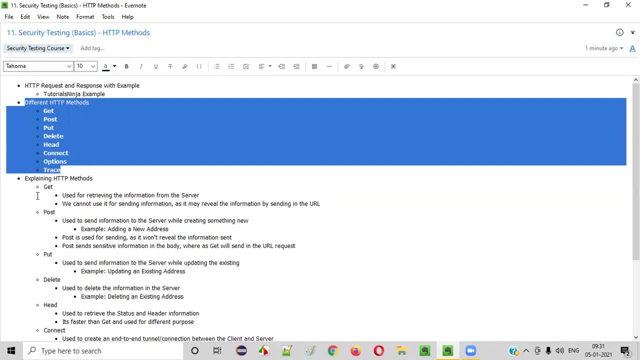 The different HTTP methods and what exactly they do, and thereafter I'll explain which out of these HTTP methods are safe and which out of these HTTP methods are dangerous in terms of security- Everything I'm going to explain, guys, in this session. So we'll start with the concept first. 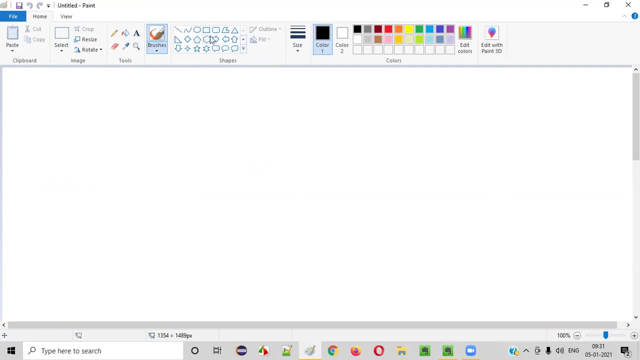 So in order to understand the HTTP methods in a better way, you need to understand this concept. So, generally, we have something like a client, guys okay, and other side we have something like a server right, a client and server like this. So let's say, the client is nothing but a machine. 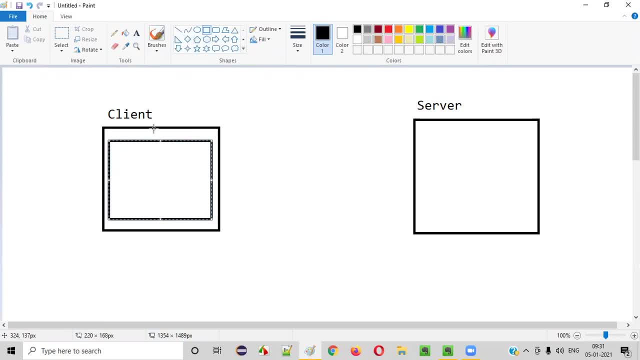 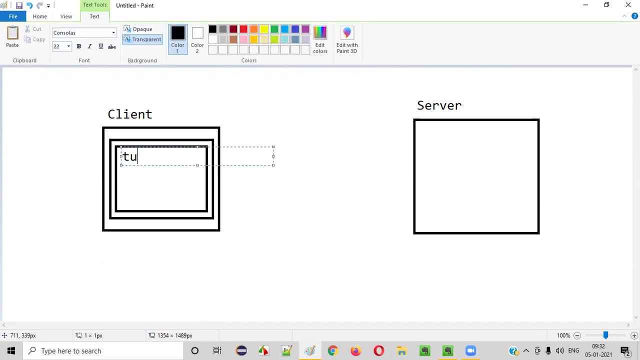 or a laptop. let's say: this is your laptop and I'm calling this laptop as a client. fine, in this laptop you have opened a browser. okay, you opened a browser and you accessed some application. let's say, you accessed some tutorials- Ninja application. let's say: okay, you accessed some tutorials in the application. 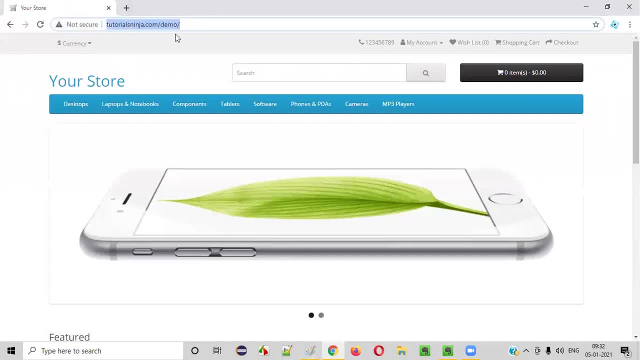 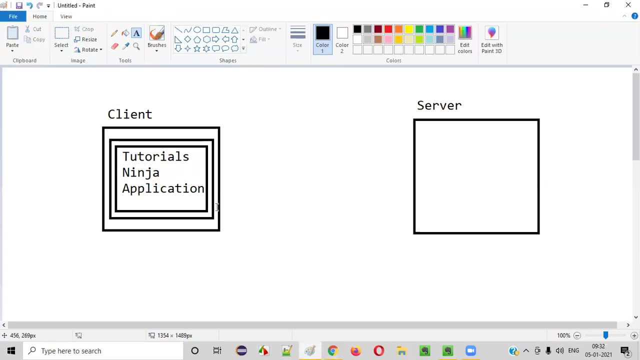 So let me show you the application. how does it look? let's say, this is the application you accessed in this one of the browser, like chrome browser in your laptop, the way I did. okay, and I'm calling this setup as a client. I'm calling this setup as a client, that's fine. 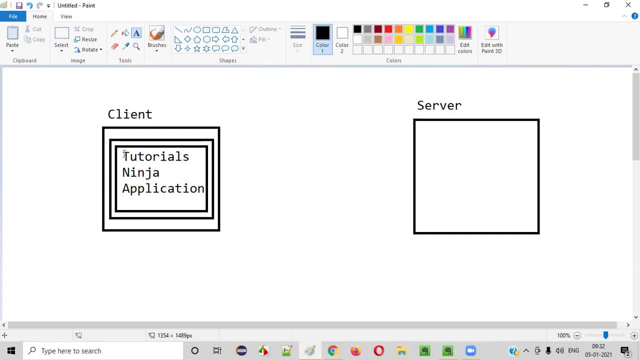 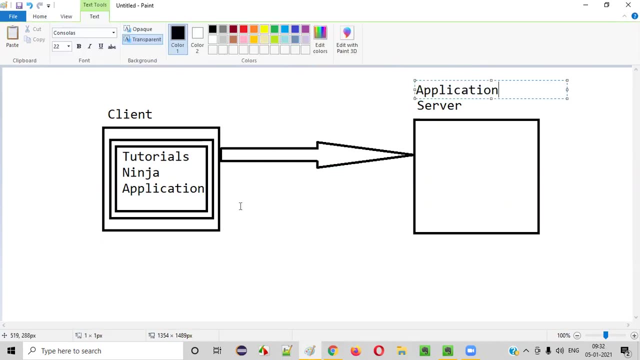 So when you open the application in this chrome browser of your laptop, what happens is a request will be sent to the server. okay, a request will be sent to the server. which server application server. So if you are using facebook application here in the client, a request will be sent to which server. 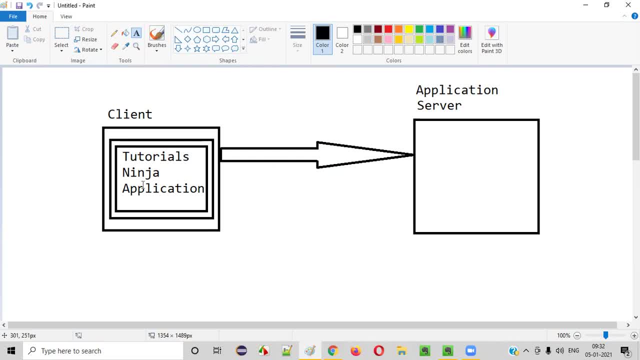 guys, facebook server. right, if you are using some amazon e-commerce application or website in your laptop for purchasing some product, then a request will be sent to which server? request will be sent to the amazon server, like that, guys. okay, I'm just explaining at a high level. 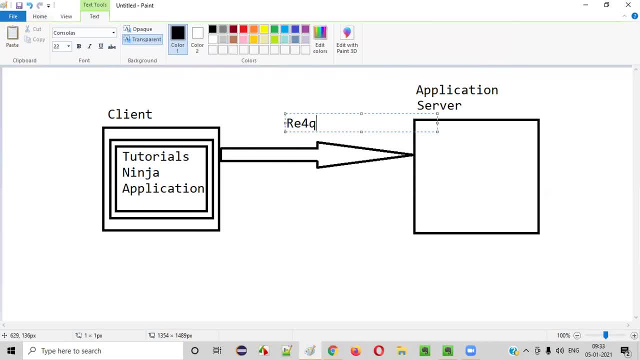 So this is nothing but the request guys. a request will be sent to the server from the client. similarly, once this request is sent to this server, here tutorials ninja application will have which server guys, tutorials ninja application server. So this request will be processed by this server. 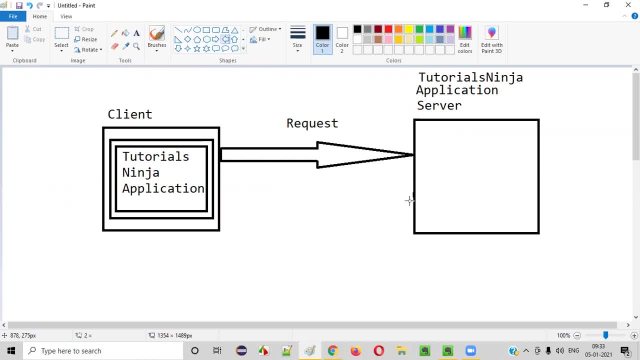 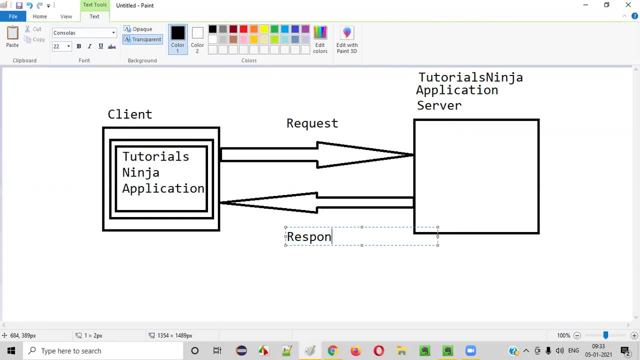 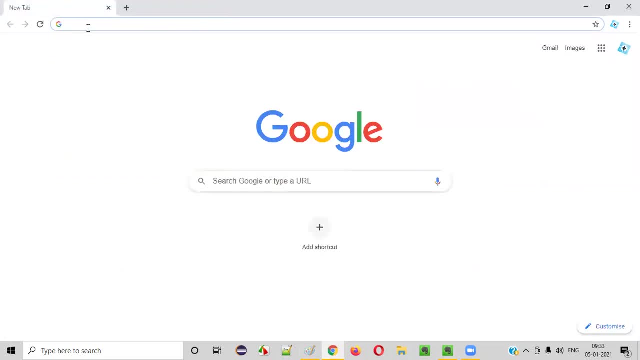 and a response will be sent back. okay, so from here, a response will be sent back by the server to the client. So this is what actually happens, guys, when you use the application right, even when you like. initially it was like this, right, my browser was like this and I don't have any url entered into this address. 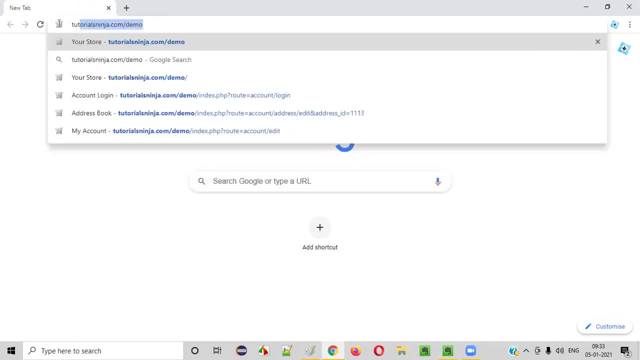 bar. so once I enter this and hit this url- okay, when I hit this url in this browser, a request will be sent from my browser. okay, to the which application server? tutorials ninja application server, a request will be sent and once that request is processed By that tutorials ninja application server, a response will be sent back and after processing. 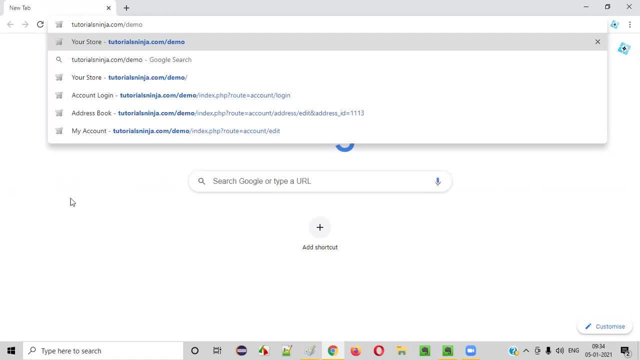 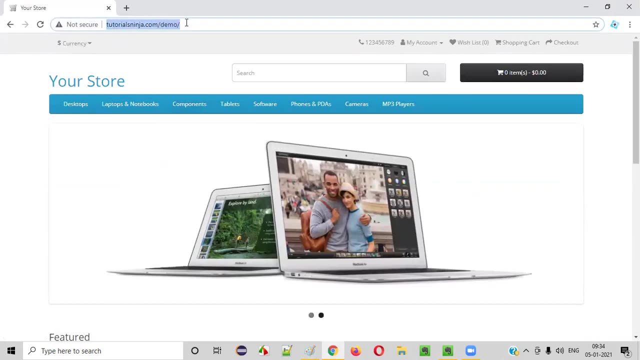 this after rendering that response: okay, your application will be displayed on this browser, guys. okay, this is what happens in the background. okay, so when you hit this url, a request is sent to the server of this application and then that application server will respond. okay, it will give. 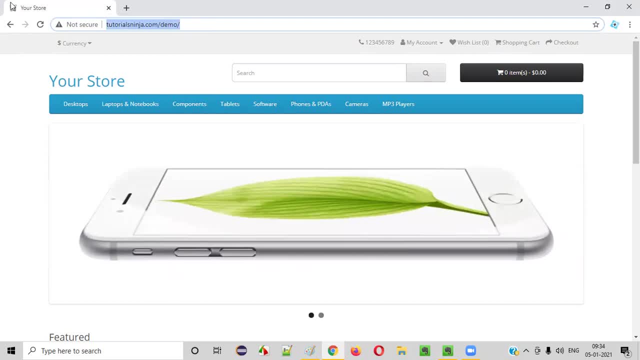 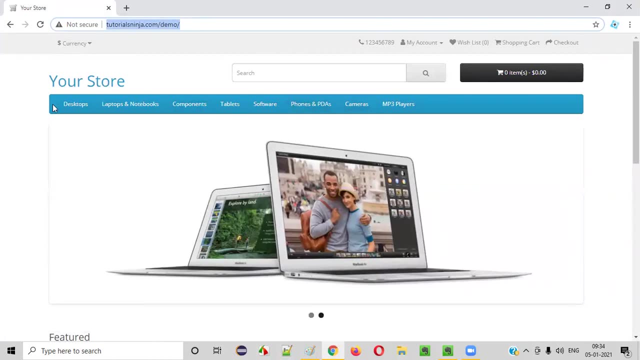 some response and, based on that response, only your browser, chrome browser, will display this particular page. So this not only just hitting the button, but also the application server will respond to the request. the browser uh url in the browser guys, all the operations. for example, if you try to create an. 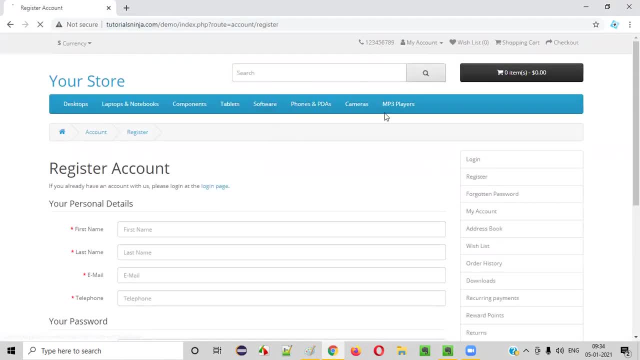 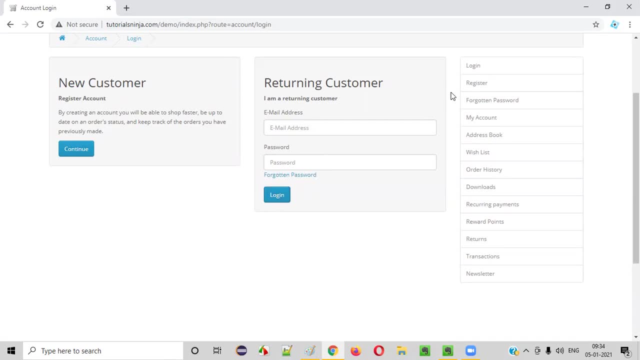 account here, okay. when you create or when you try to log in here, okay. when you give the valid credentials- or whatever the things- invalid or valid credentials- and click on the login button right, a request will be sent to the application server. it will be processed. okay and a response. 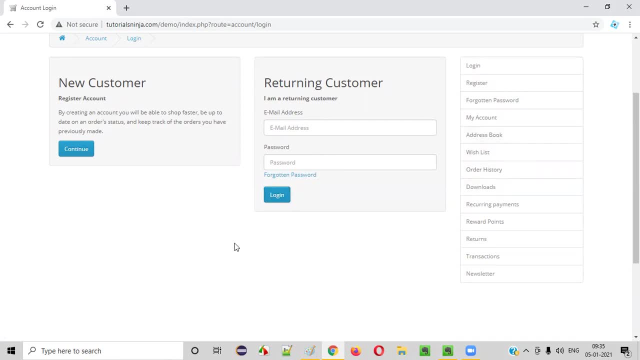 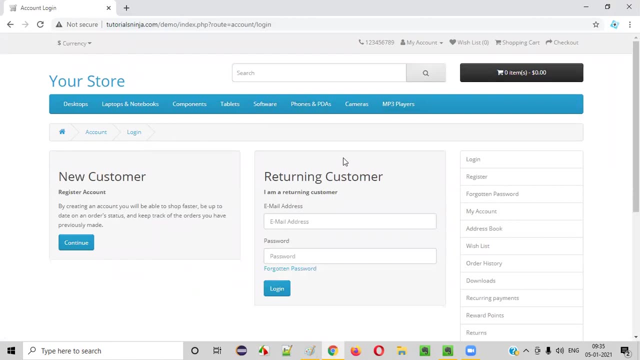 will be sent back to the application, this browser, and if the response is proper, only then only you will be able to log in in this browser. otherwise you'll not be able to log in. fine, so like that, guys, everything is a request and response between the client and server, your application, and. 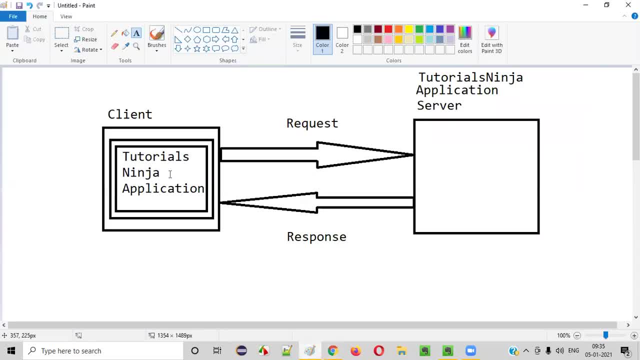 application server. some communication will happen like request and response, like this, guys, fine, so let me show you practically what exactly happens. okay, how does the request look and how does the response look? i'll take an example and tell you now. okay, fine, so i'll open this empty browser. 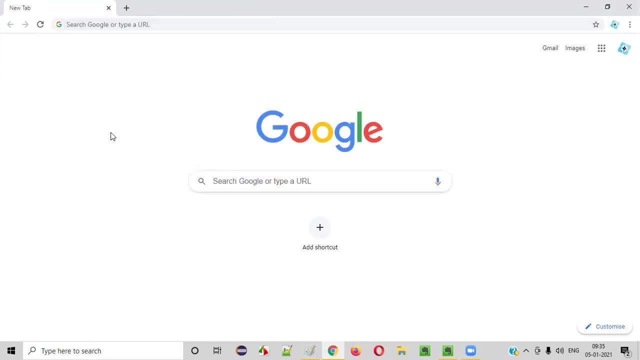 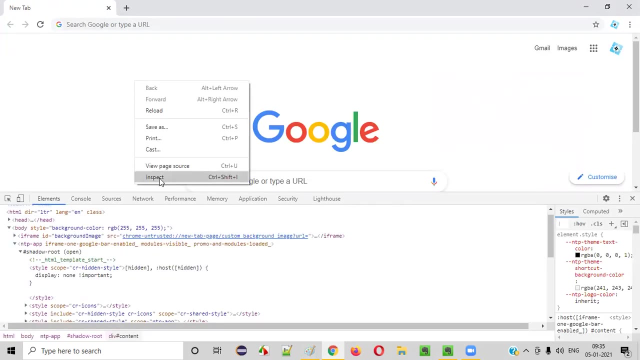 and here, before hitting any url, what i want to do is: i'll right click and inspect, guys. okay, i'll right click and inspect this and once i uh, right click and inspect. uh, if you are getting this kind of thing here, that's fine. otherwise you can. 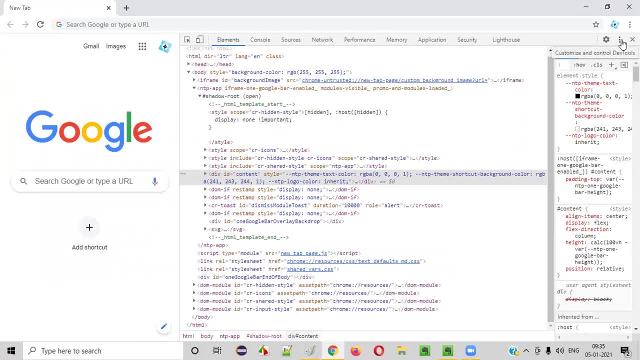 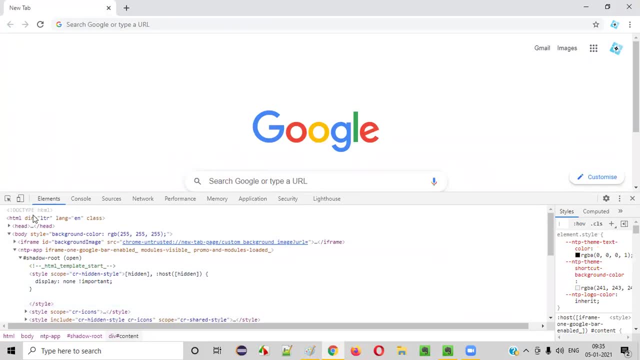 change the orientation here. so, for example, if it is like this for you in the initial, so simply change it to like this, okay, then you will get this kind of dog thing in the bottom of the page. now, by default. which tab is selected in this? uh, chrome developer options- elements- elements tab. 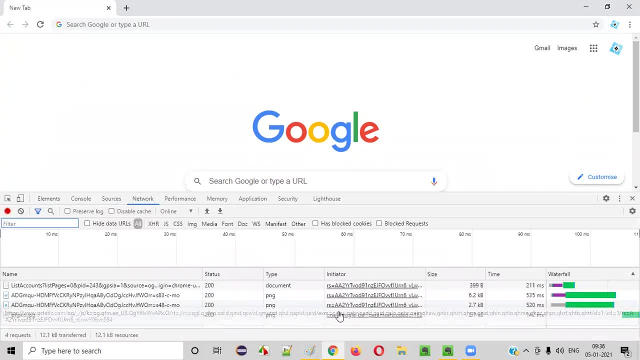 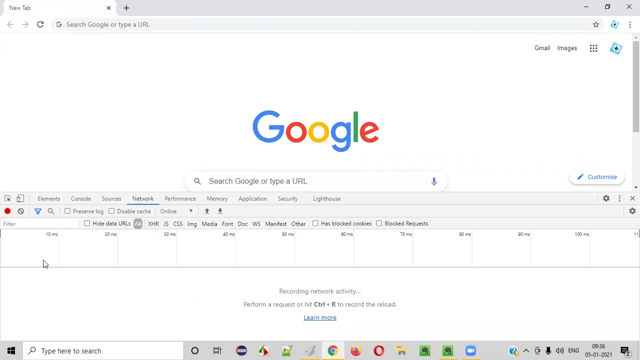 right, i need to select the network tab. okay, for this purpose, to understand this uh request and response between the client and server, you need to select this network tab. so there are already something there. you can clear it out. okay, you don't have to uh watch the earlier ones. so once uh, there is nothing here. once you have cleared up, clear it. 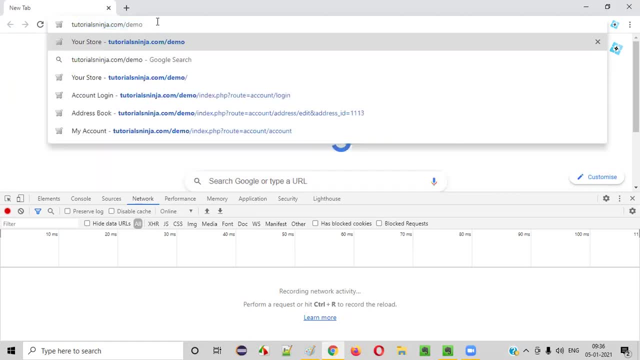 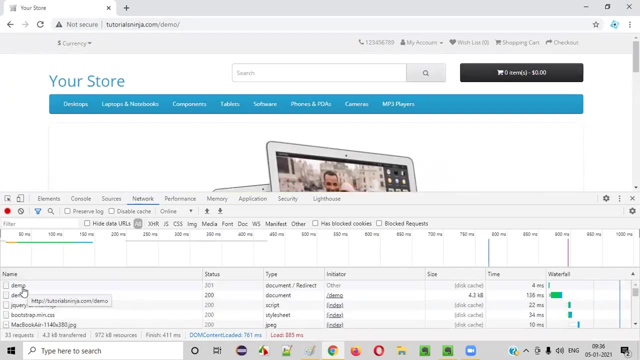 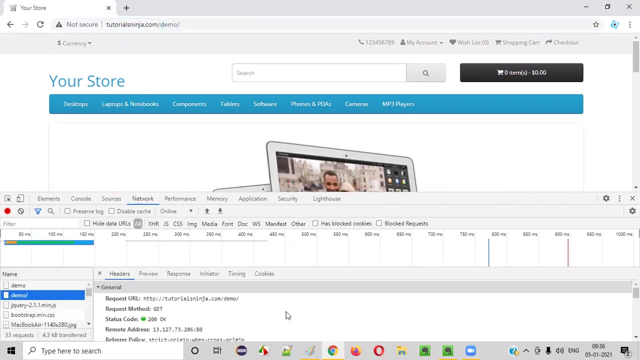 out. simply hit this url. guys. tutorials, ninjacom, demo. hit this url in the browser. when you hit the url, you see something happened here, right, some? uh, there was nothing here and you see something like demo, demo slash and all the stuff. so this one is like demo slash. i'll go with this demo slash. 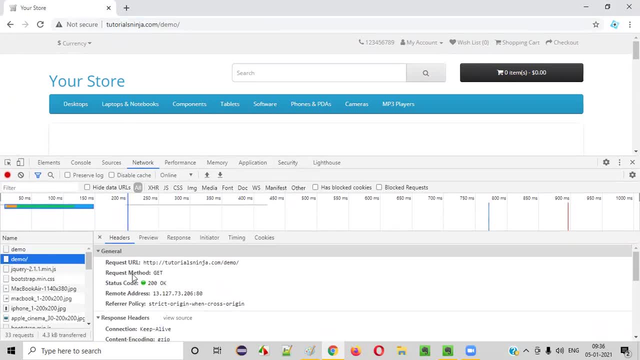 and see here this, this, uh. these options give you clear picture like a request has been sent. okay, when you hit this particular url in this chrome browser, your chrome browser has sent a request. okay, a request has been sent. so what is the request? request is nothing but the url of this application, guys, that. 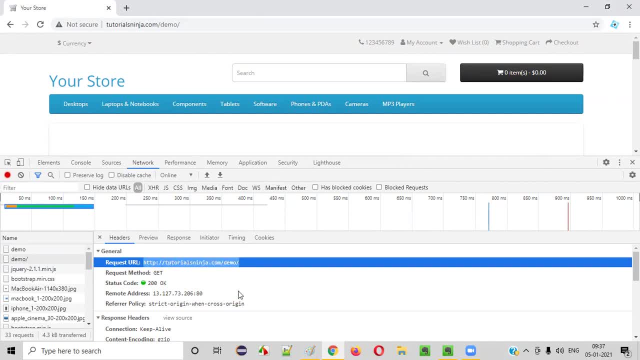 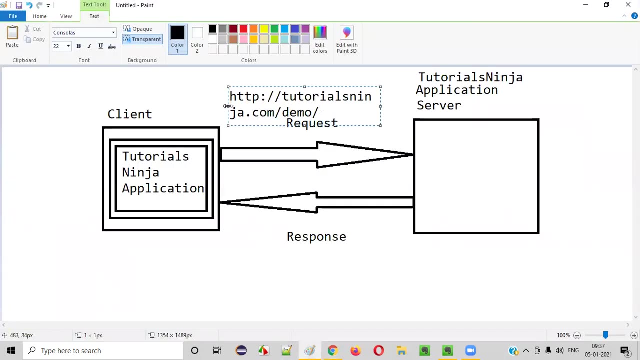 is tutorialscom demo sent as a request? okay, this particular thing has been sent as a request. so what is the request? is nothing but the request. http//tutorialsingercom slash demo is a request. this request has been. request will have the url, guys. okay, so a url has been sent to the server. application server once. 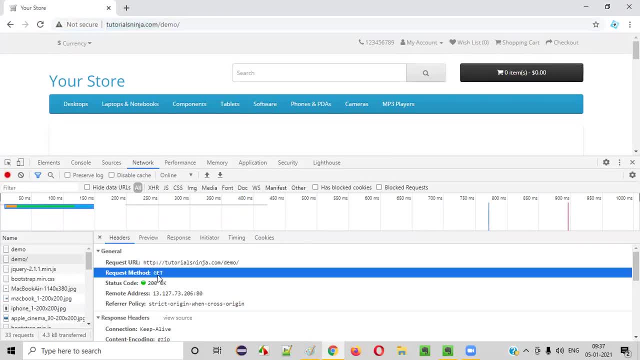 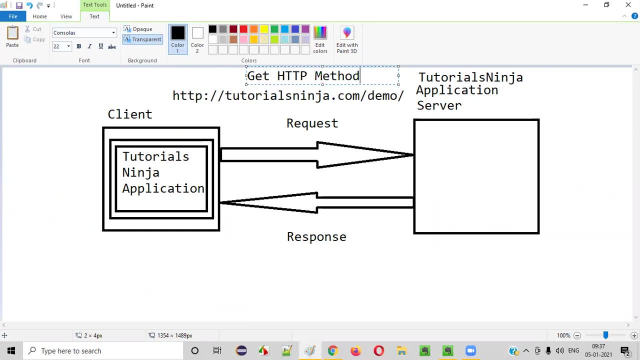 this request has been sent. so here one more thing is observed. this: you see, there is a get kind of method. okay, http method is used. which which type of http method is used by this request? some get method. okay, here, get http method is used. i will explain why get http method is used in this. 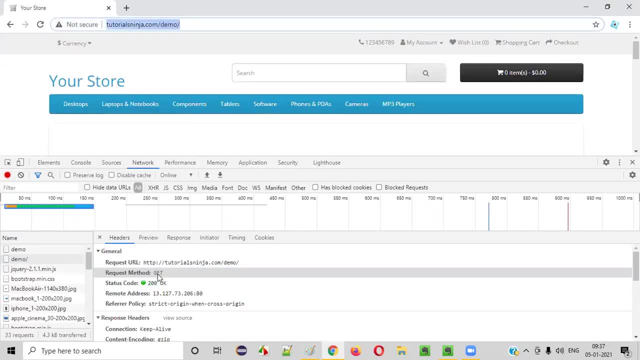 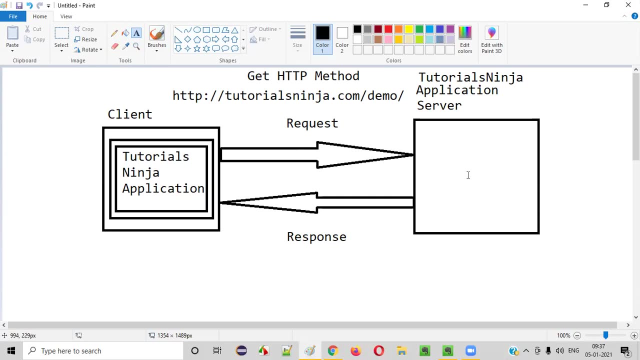 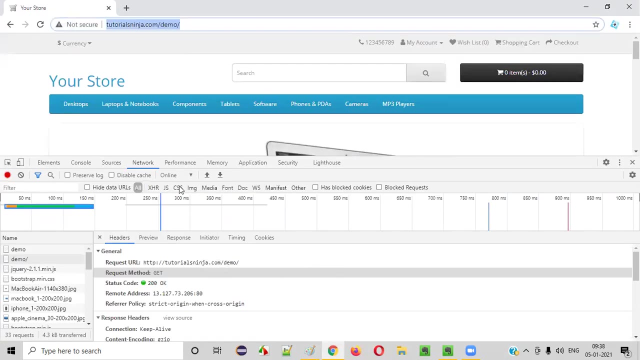 in this kind of example, why get http request method is used. i will explain later. fine, fine, so a get http method with this url has been sent to the application server. application server will process this and will respond something. so what will be the response? the response is nothing, but this is the response. so, apart from the headers, 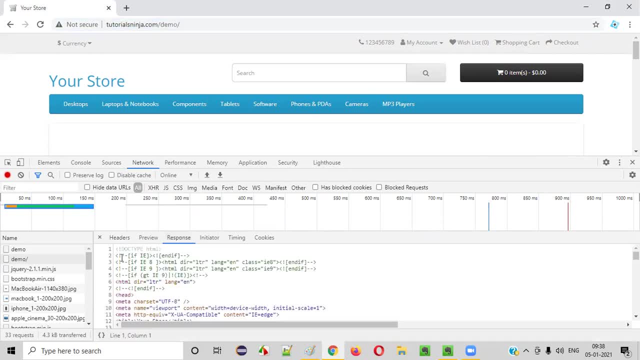 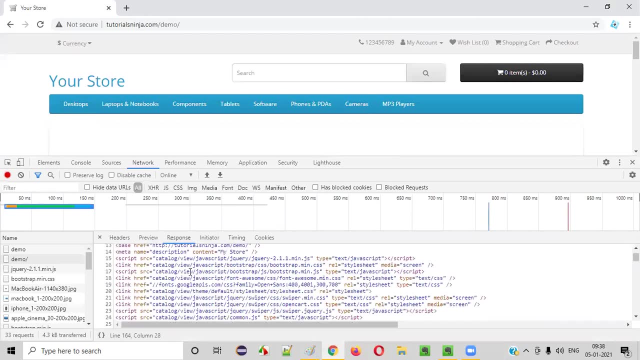 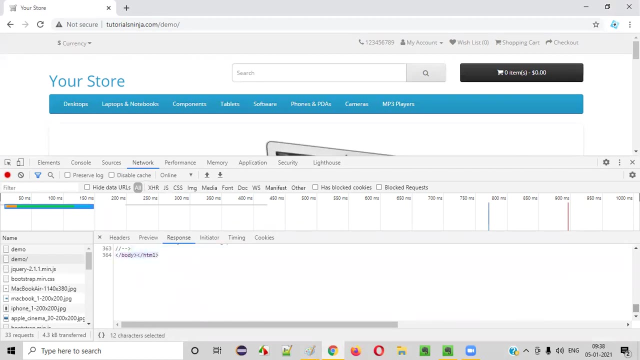 here. you have this response also here. right click on this response. so this has come in the response. okay, this has come in the response. what is actually there in the response, guys? some html code is there. okay, this response has a html code. you see, the ending is like a body html. this is like html code. 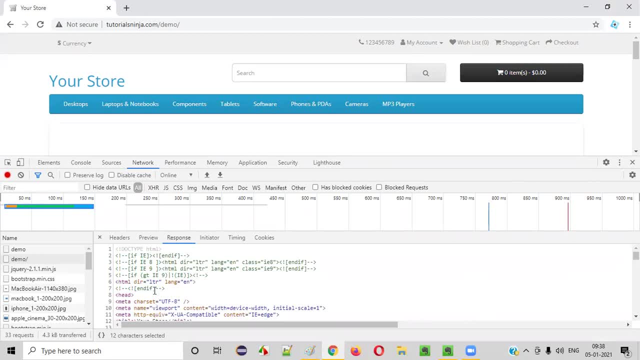 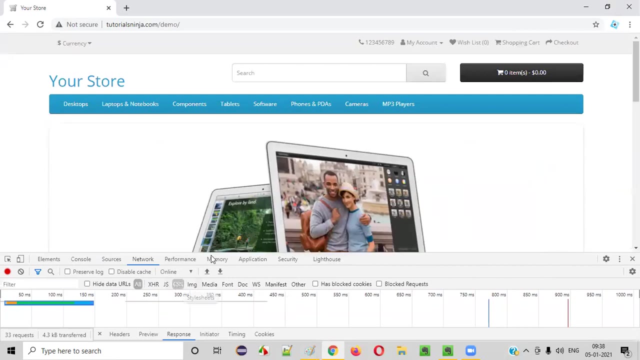 right, so some html code is coming in the response from the server. this html code will be main processed by this browser in your client machine and, according to the html code that has come as a response, we'll see this page. okay, this page is nothing, but whatever the 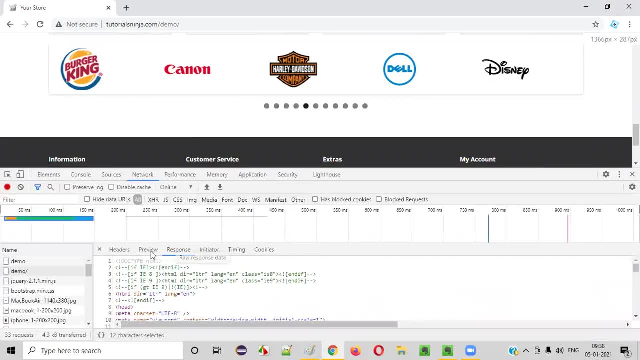 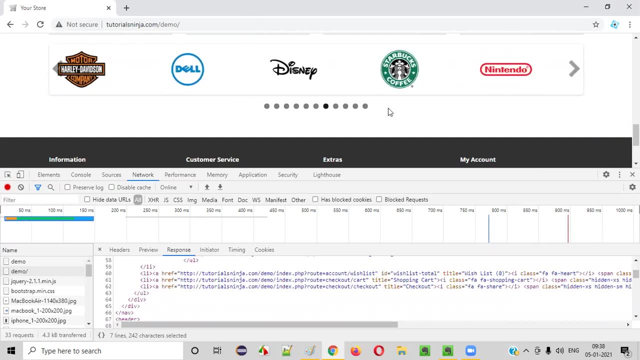 ui. that you see on this page is nothing but the rendering of the html code which came from the server. okay, this html code is rendered on this browser, but this html code came from where guys? from the application server. okay, from the application server, you got this html code. 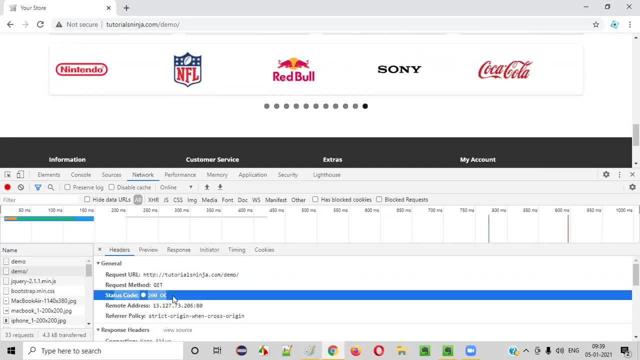 and along with this html code, you also got the status code, guys. okay, whether this html code is your request is successful or not, i'll explain more about the status codes in the next session, guys. for now, let's focus more on this. http methods, okay, so, anyhow. so, as a response, what we got, guys. 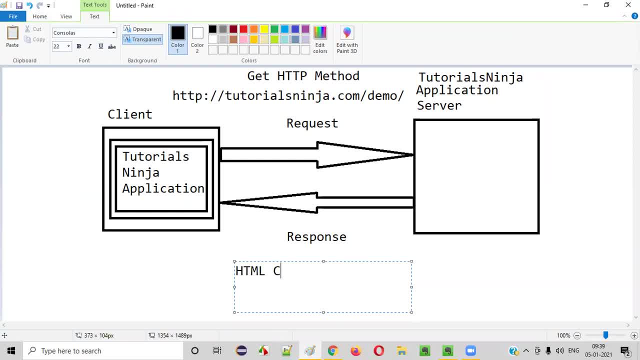 at a high level at the response. we got some html code, we got in the response and along with that we we got the status code like 200 okay and that kind of thing. so if everything- this request and response- is okay, right, you will get the status code as 200 okay or something. so, uh, what's the? 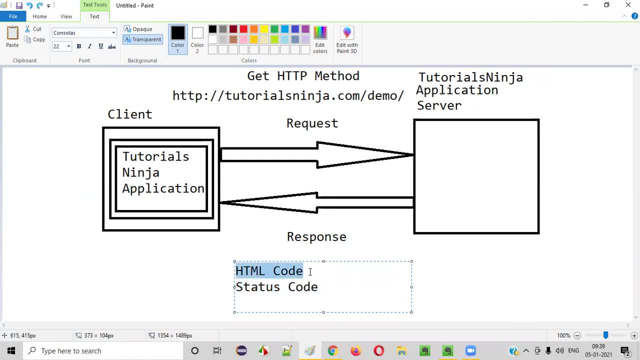 should be displayed on the page that will be coming as a response. html code- response: fine, this html code will be used by the browser of this client machine to display the page properly. fine, so this is at a high level, guys, concept. now let's move into the details. so the next thing is: 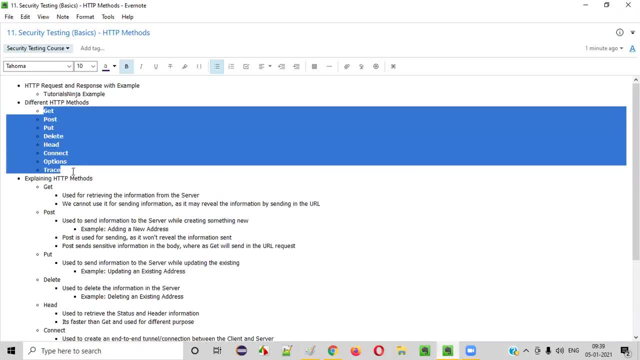 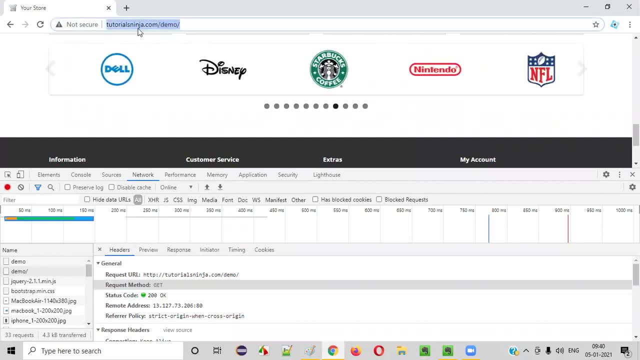 like, once you understand this concept. there are several http methods in this example, guys, the http method that was used by this- uh okay, request. when you hit the application url, which http was used for sending this as a request to the server? the git you see. you can see here: get. 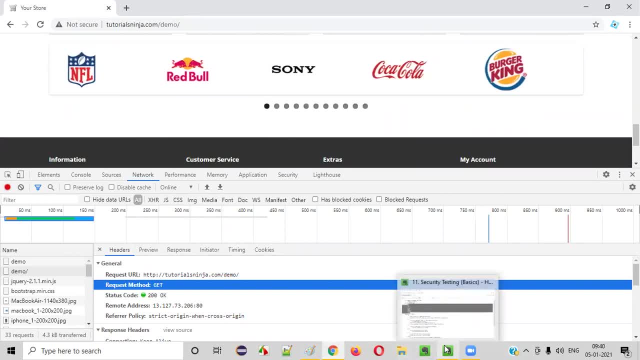 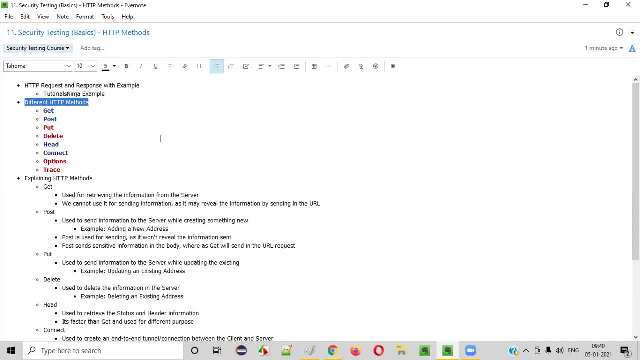 get is there. this was used. why it is used, i will explain now, anyhow, but before i explain why get is used, i'll explain one more thing. so here there are different http methods, guys. okay, not only get. whatever you see in this example is only get. but apart from get, there are several other http methods. 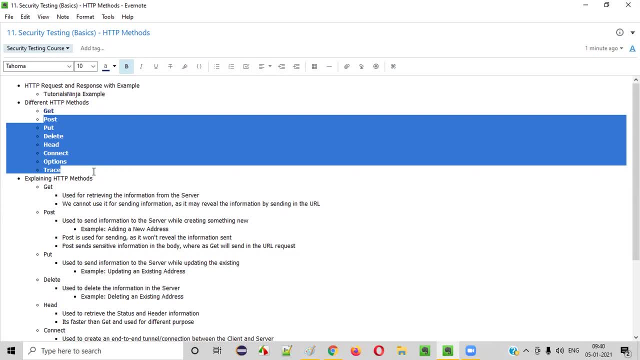 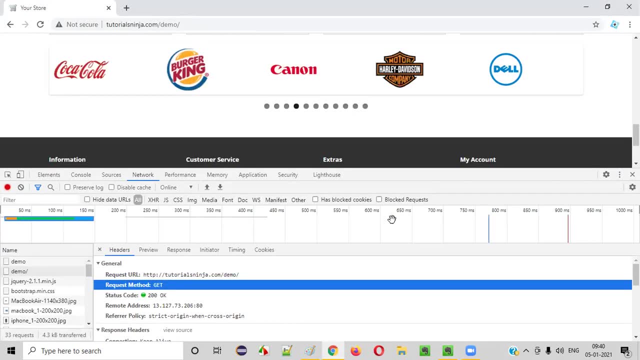 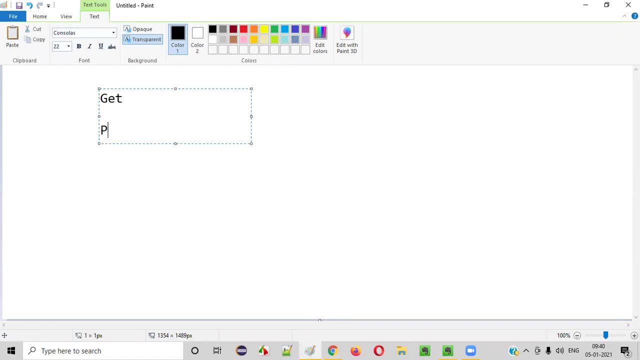 okay, that will be used by your application in your client machine to while sending the request to the server. fine, so, anyhow, what are the different http methods we have? let's list on them. so for now we have known one thing is get right. then we have post. 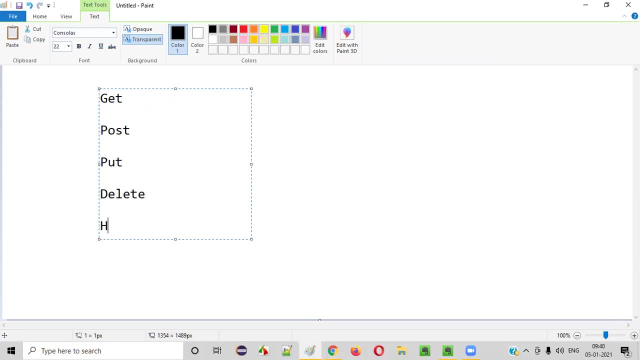 then we have put, then we have delete, then we have head, then we have options, then we have trace. okay, so head options phrase. any other thing left out? yeah, connect, is there one or another thing is connect, head connect. so i'll just remove the spaces so that 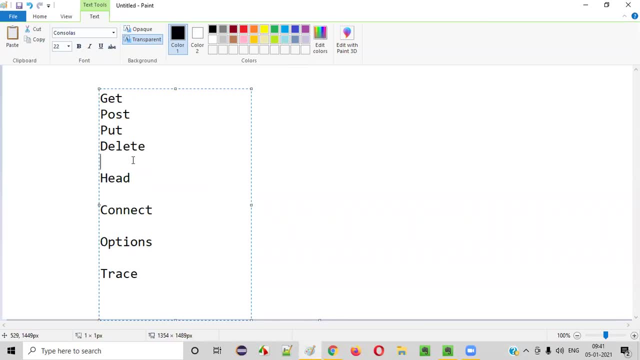 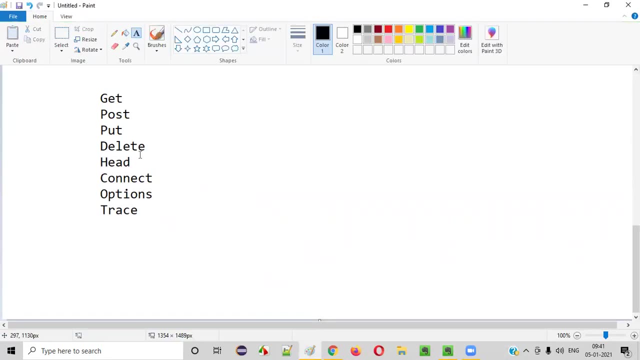 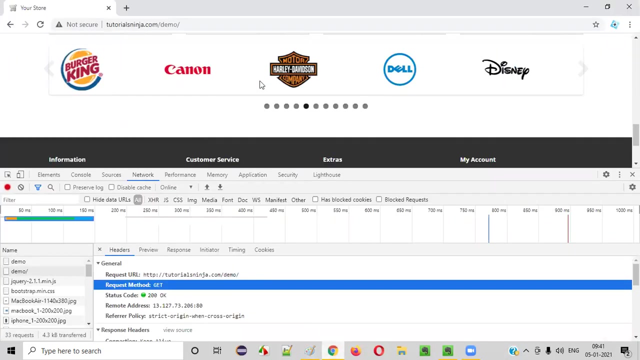 you can see everything in a single place: get post, put delete, head right, connect options and trace. these are all the different different http methods. okay, these are all the different http methods. so in our example, in our first example, the first uh http method was like: get right, so why get? 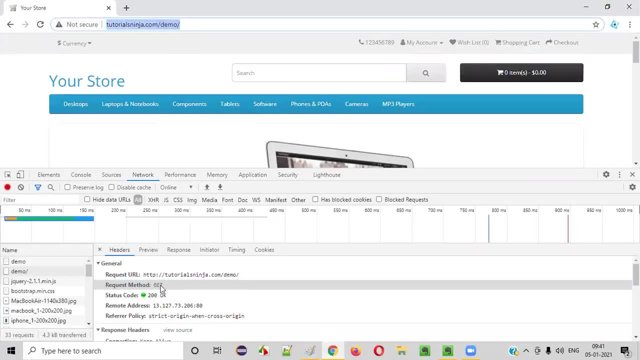 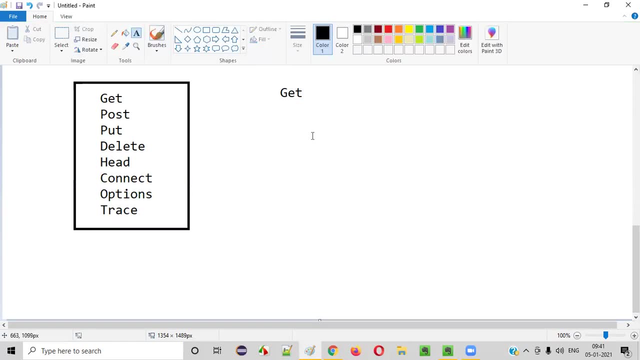 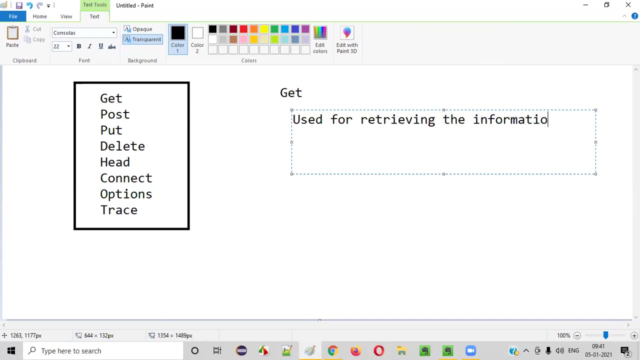 was used in this kind of situation when you hit the url. why get was used as part of the http method while sending the request to the server? the answer here is: get is for is generally used for retrieving the information from the server in all the cases where you have to get the. 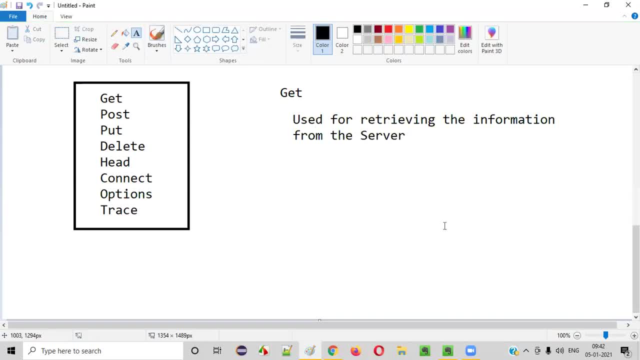 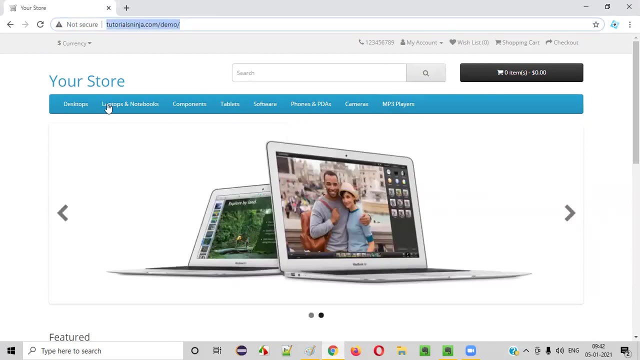 information from the server guys, then we have to, then the developers generally code this: get, get http method while sending the request to the server guys. fine, so here, what information we are getting when you hit this url. what you are getting guys, the response, what information you are getting. you are getting the application page right. this is. 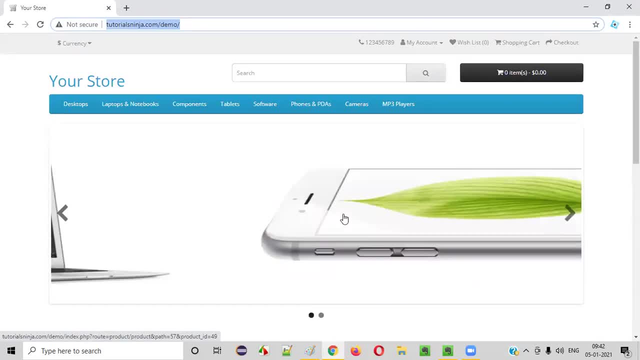 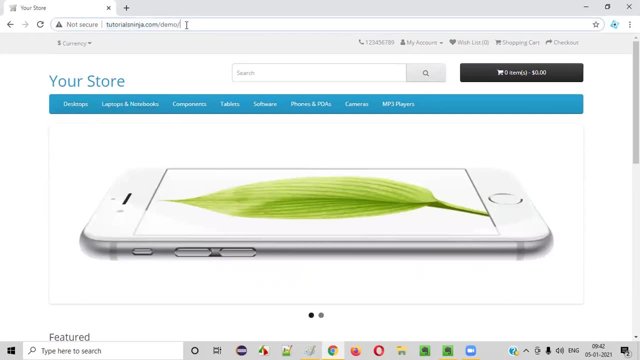 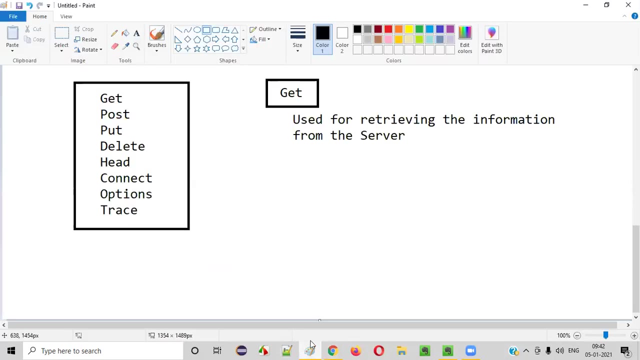 just an information. you are not submitting any information. you are instead getting some information like: uh, you are getting this home page and all those stuff, fine, so get is used in all the places where you retrieve the information from the server. so, uh, one more thing like for. 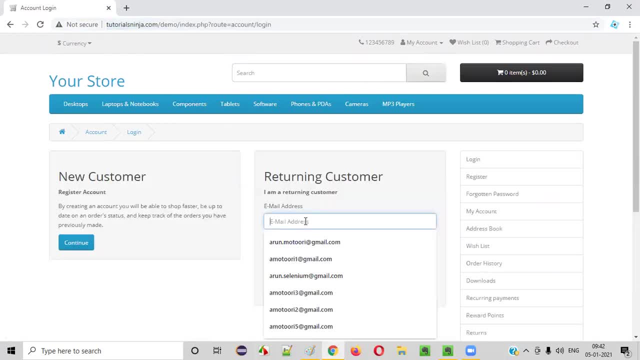 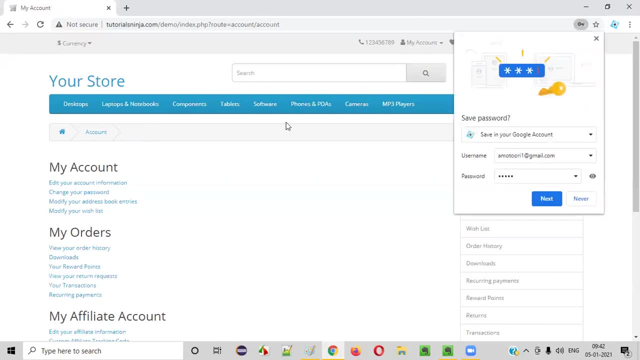 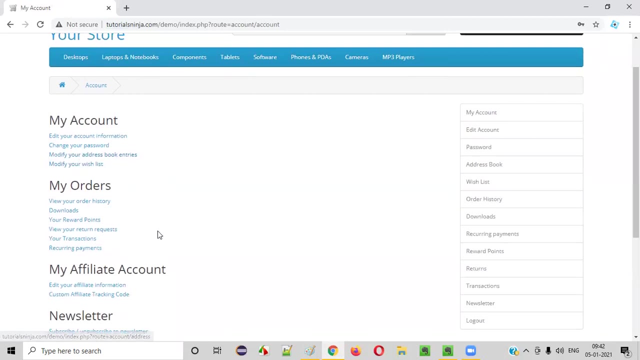 example. i'll take one more example for the gate guys, so if i log into this application, if i log into this application, one, two, three, four, five login. and here, guys, so if i click on any of these options, like, for example, if i click on- uh, what do you call manage your address book entries? when i click on 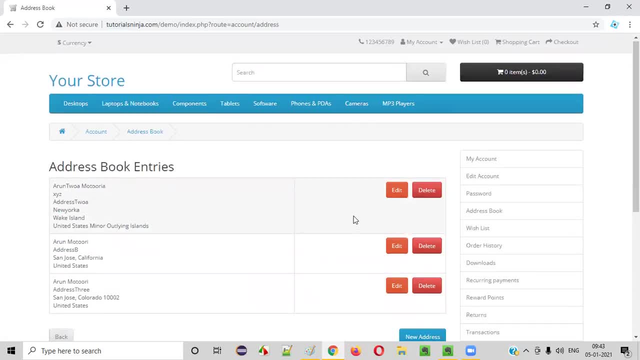 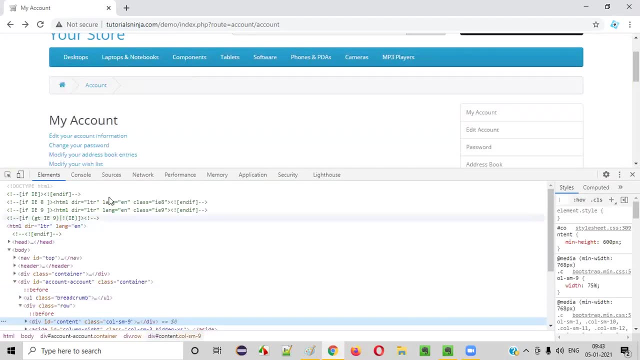 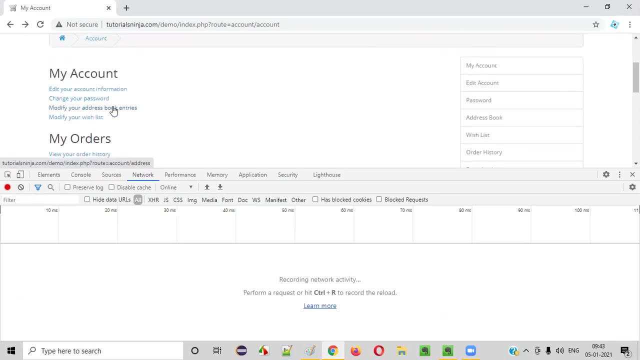 this automatically. a get request will be placed here, guys, and you will see all this address. okay, so let me do one thing. i'll inspect this and i'll go to the network tab and i'll clear all the previous things and simply click on this. modify your address book entries option. 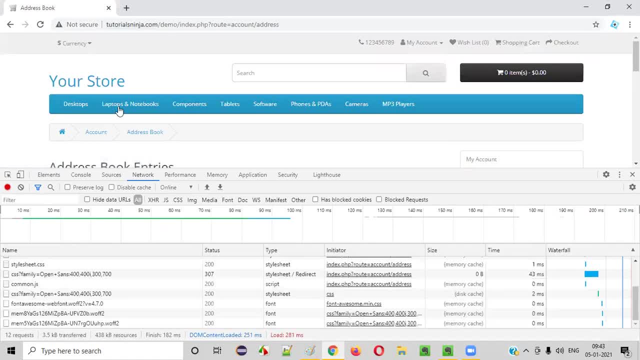 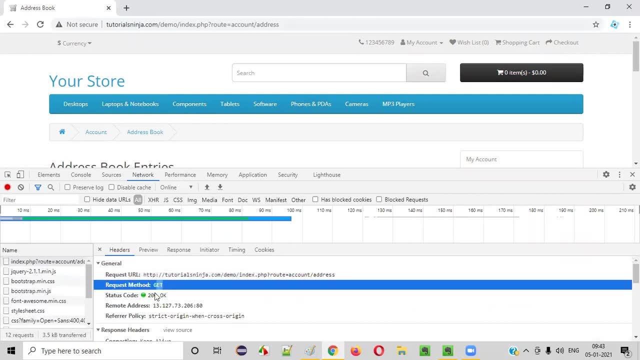 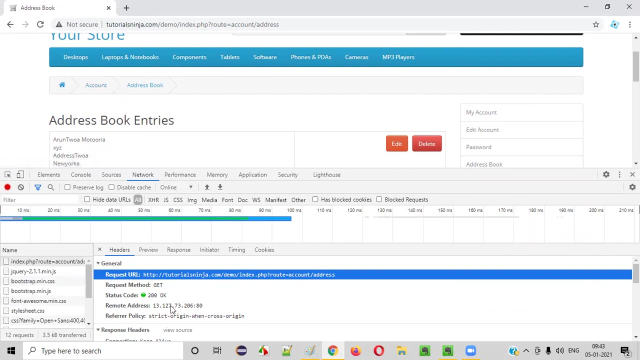 in this, my account page. when i do that you see some some address related stuff is there here. get is there? why get? is there? a request has been sent. when you click on that address link address, kind of link option in the account page, the moment i click a url request has been. a request has been. 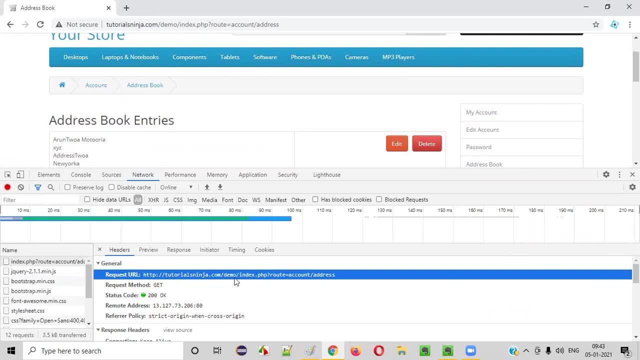 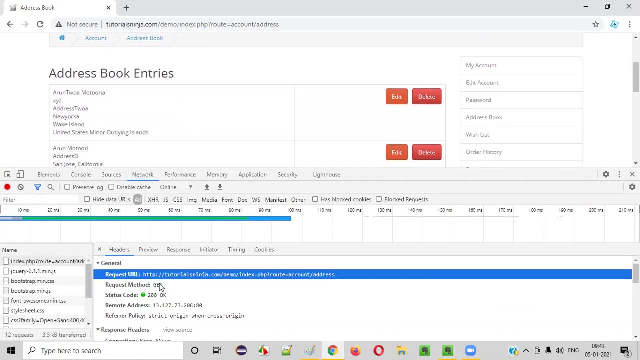 sent to the server guys with this url, that is, tutorials, ninjacom, slash demo, slash. indexphp. root is equal to account slash address and, along with this url, what type of request method has been used? http method, http request method? get why? because using this url and get request method, get okay, get http request method. we are retrieving all. 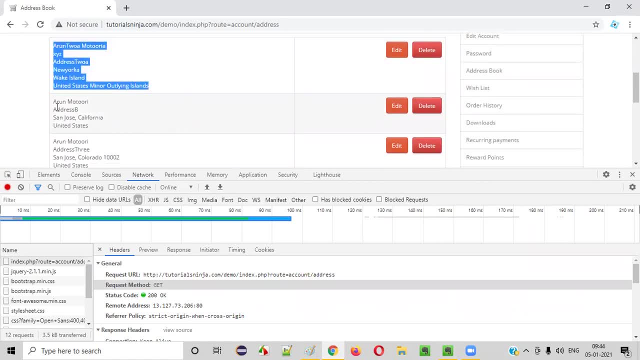 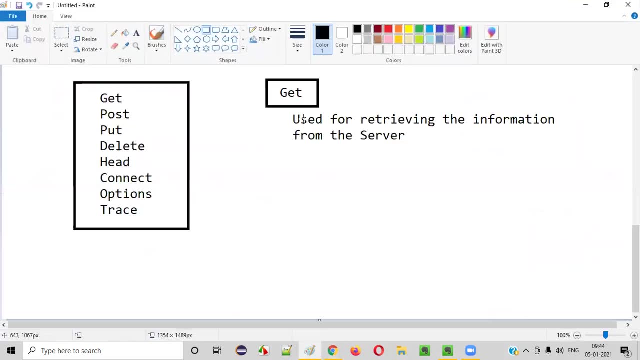 this information from the server. you see, all the existing addresses that are already stored in the application server are getting displayed here. this is what information we are getting, guys. that is the purpose of the gate. okay, hope you understood what's get is used for in all the 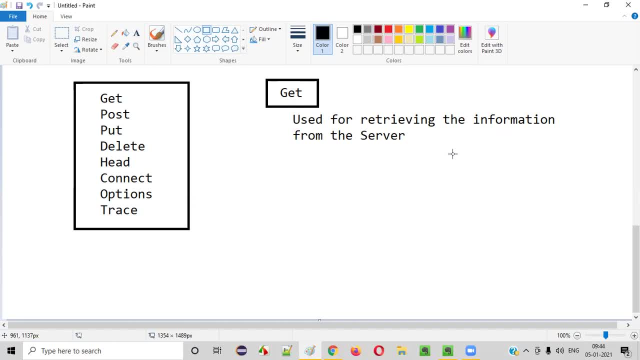 places of the application where you have to retrieve the information. okay, when you click on some link or something and it if it has to fetch some information. or if you click on some button, also okay. sometimes, when we, let's say, view all the employees in the company, some button is there if you click on that. that request has to be sent to the server server. 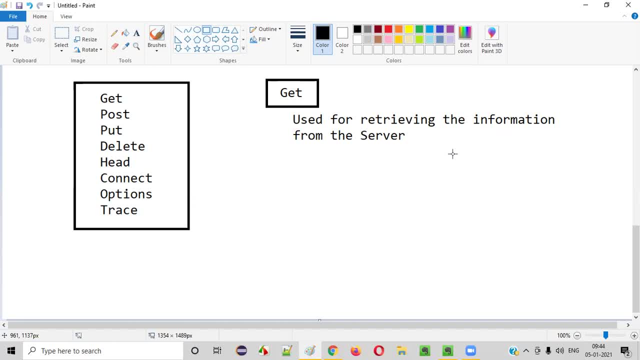 has sent all the employee details that are working, who are working in the company, on that displayed on the page. so in that case also, which method will be used. get method will be used for retrieving the information. we have to use a get method, then we'll go with the next method, guys, that is, post. 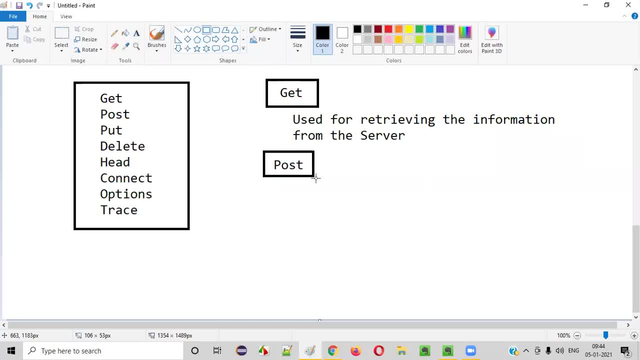 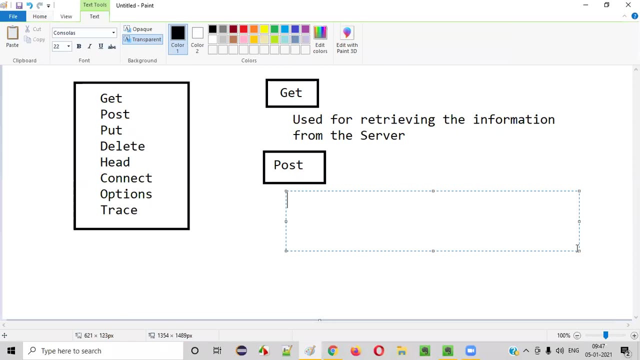 okay, post method. the second method is post method. so what is this post method? post method is used for sending the information, guys, unlike get method. get http method was used for retrieving the information from the server, whereas post is used for reverse guys, that is used for sending the information to the server. okay, to the server, if you are sending the information. 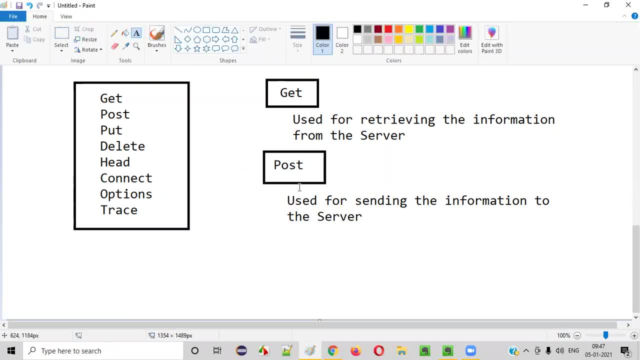 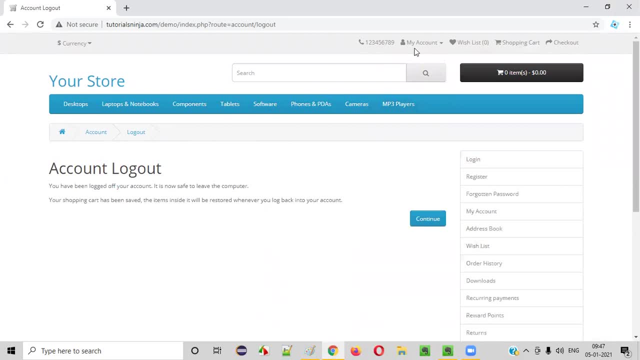 then we'll be using post. fine, so let me give some examples where exactly we use post. i'll take the real examples, i'll just log it out. so in this application guys, for example, if i go to this uh register page, let's say i'm going to 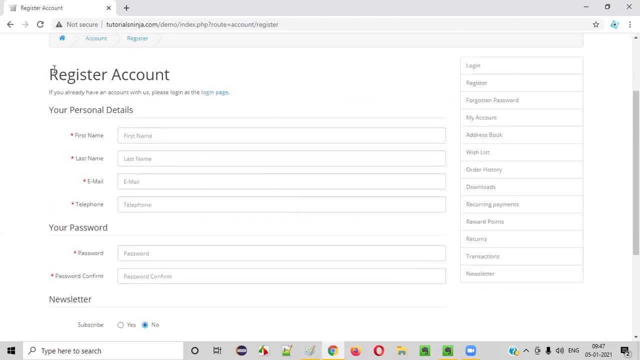 if i have. if you have to create an account here, okay. if you have to register a new account here, create a new account. then for this we will use post. okay, post will be used here because, uh, you are sending the information to the server and asking the server to create an account, with all. 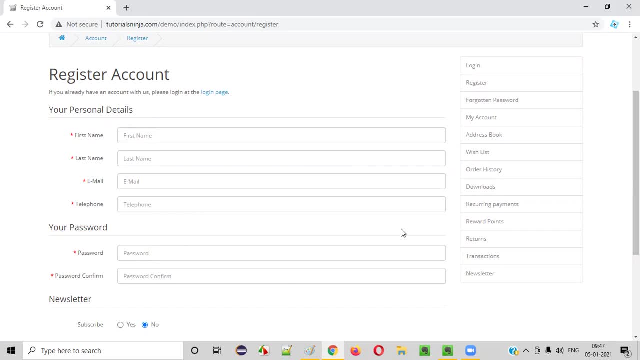 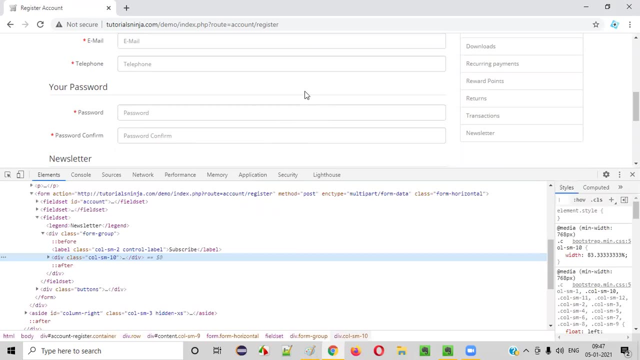 the details that you are sending to the server. that's what is a post all about, guys. okay, so here, when you, when someone clicks on this- i will not fill any details here, but i will show you at a high level. okay, so here i'll go to the network tab again and clear the things and here 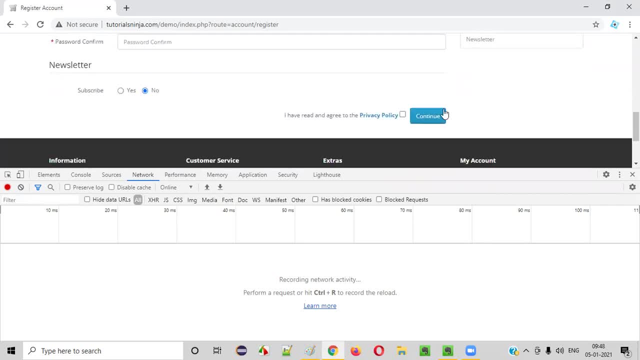 i'll simply click on the continue button. guys, whether you fill the details or without filling the details, if you click on the continue button, the same request will be placed. fine, so i'm just clicking on the continue button. the moment i click on the continue button, i got this. uh, okay, this is. 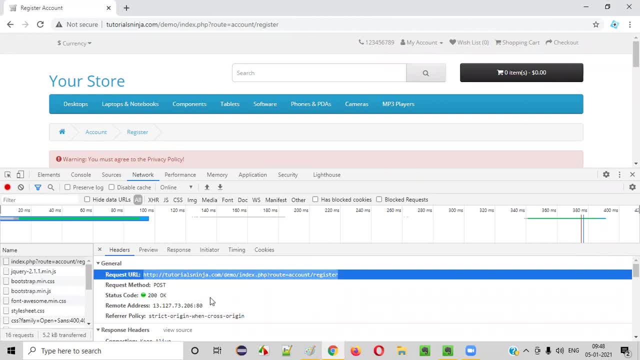 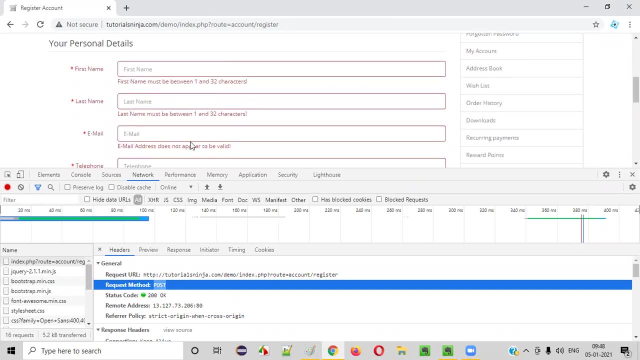 a. this is a request url that has been sent to the server, and what type of http method was used here? post. the reason here is here. you are going to send some information to the server. okay, in case of you sending some information to the server, then the application developers will use this post method, guys, okay, post method. 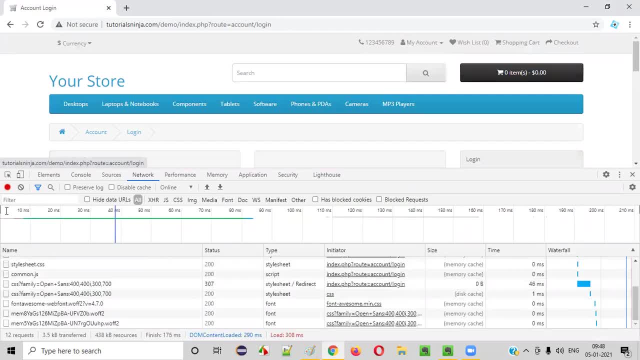 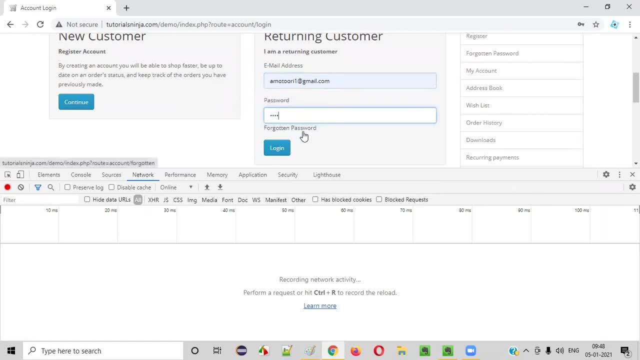 not only this one, guys. for example, if you go to this login page, also, the same thing is there. clear this out now. if i give some credentials, okay, if i enter some credentials and click on the login button here, a request will be sent to the server with the details. okay, these details. 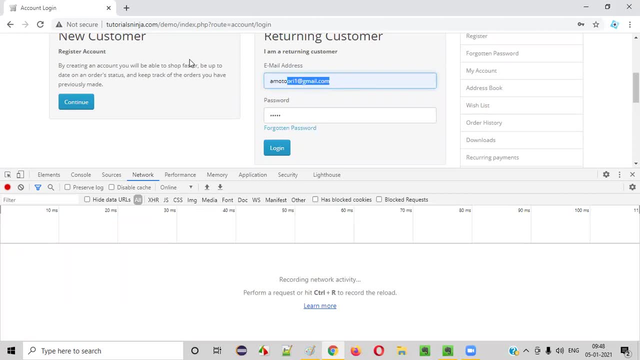 need to be sent to the server. guys, right? whatever the details and email address and password, i am giving right, these details need to be sent to the server. for sending the information to the server, which http method need to be used? post guys, login now. go here and see. 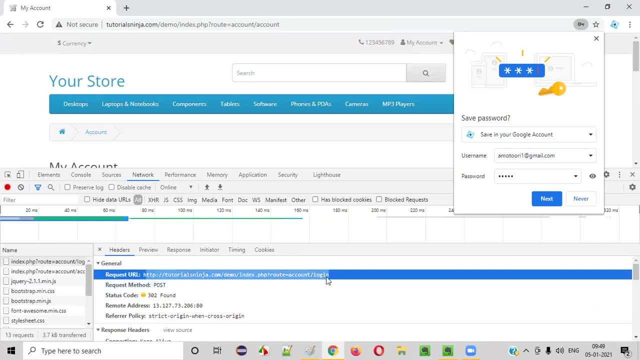 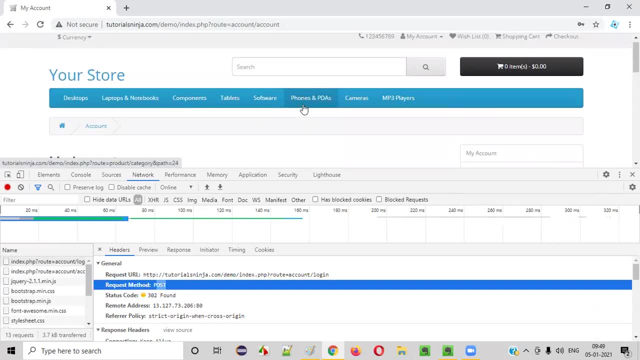 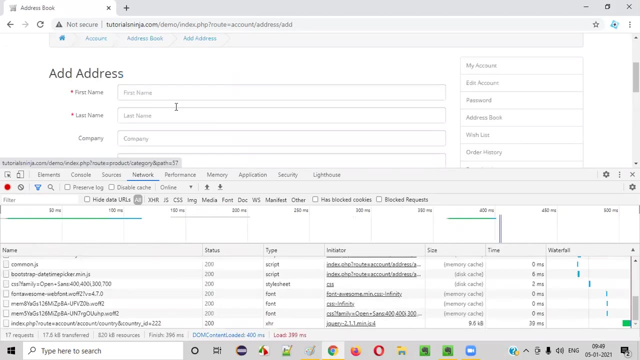 you see, this is a request request url that has been sent to the server, and what is the type of the method post? so, so, wherever you see this kind of forms, guys, wherever you like. for example, if i go to this manage address book, if i click on this uh, new address, okay here, this kind of forms you see, right. 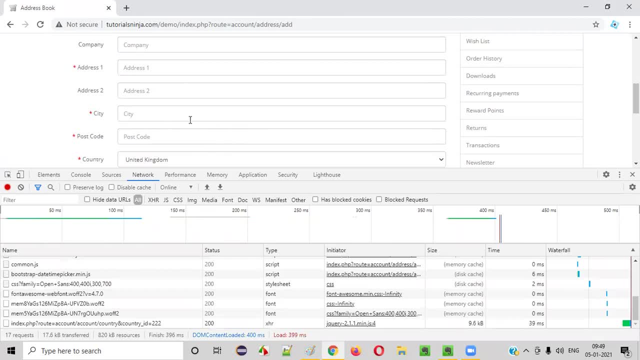 with some continue buttons, right, in all these cases, some information will need to be passed to the server and server. okay, uh, in that kind of case, guys, if the information need to be sent to the server, then we need to use some method, http method, known as post post. http method will be used in all. 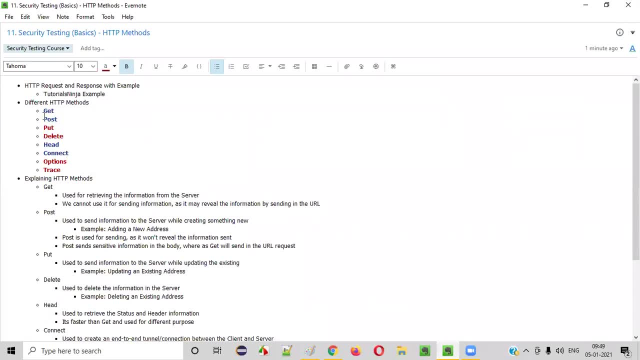 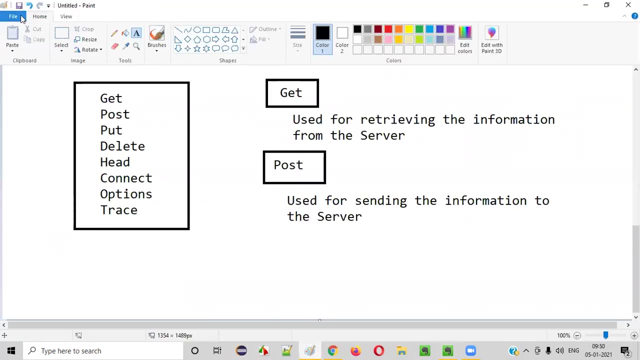 these cases. so hope you understood. uh, what is uh get and what is post? that's fine, but which one is secure? guys out of get and post? why not get? why not get is not used for uh sending the information, okay, so what's the difference actually, in terms of security? i'm talking here. so now you understood. 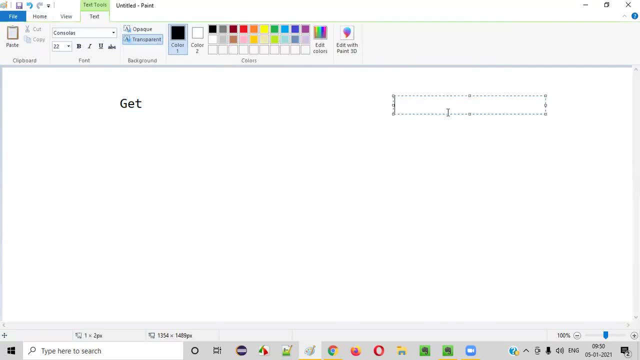 what is get and post now, in terms of security, which one is better? while sending the information, get our post. so if you use the get- okay, get- for sending the information, then what happens is get will be sent. get will be sending that information in the form of the url. okay, as part of the url, get will be sending the information, okay. 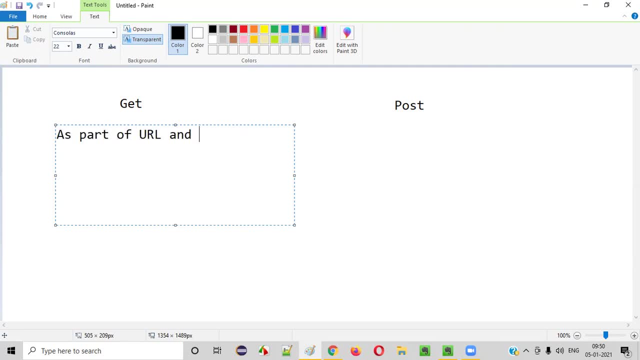 as part of url and its parameters, get will be sending the information. we can even use get for sending the information, guys, but if you use a get for sending the information, all the details that you are entering, right- your first name, last name, or email address or password, whatever it is- that need to be sent as. 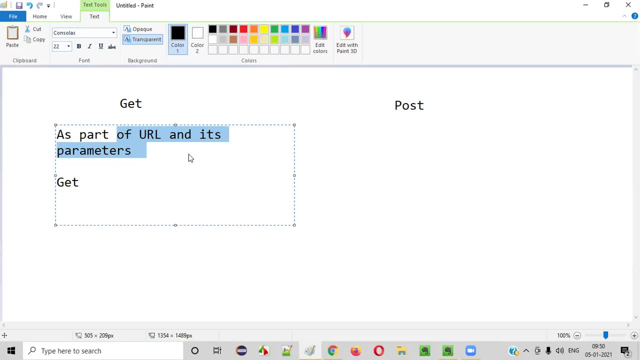 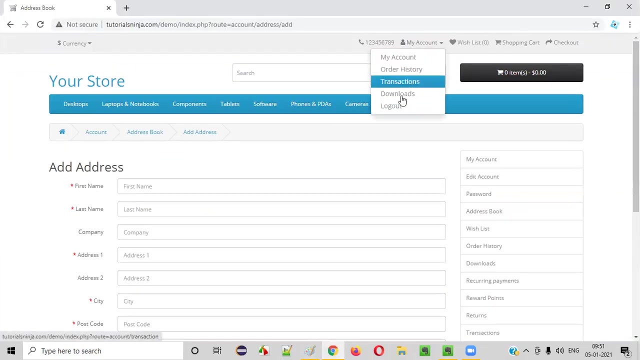 part of the url, guys. in the url, the username and password will be displayed. okay. so if you use get for sending the information, what is the problem, guys, in terms of security? the problem is your. for example, if you use get for- uh, this login, login purpose, let's say okay. if you use the get for 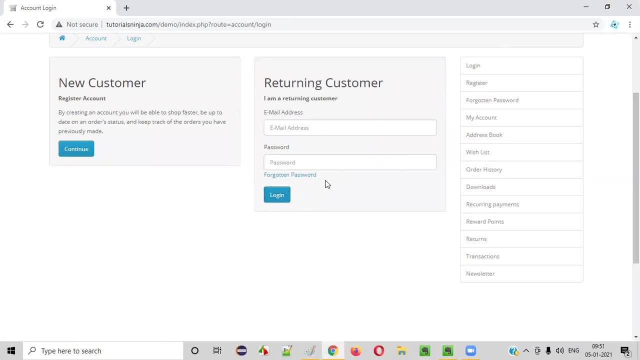 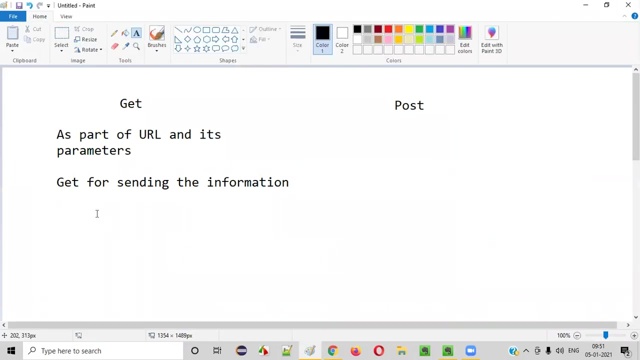 login purpose instead of post http method. if a get http method was used, when you click on the login after you enter the credentials, okay, what happens is in that get request url, this email address and password will be visible. that is a security problem. okay, your sensitive data will be exposed in the url. request url. if 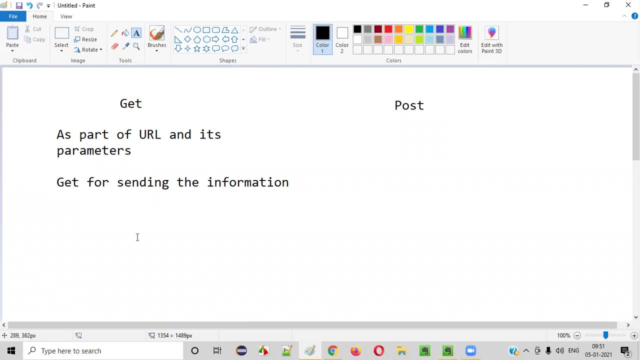 you send the email address and password that you have used for login to the application, then that sensitive information like email address and password will be visible in the url. that's why get is not generally used for sending the information to the server. so what about post, then? how the post manages this problem in terms of security. so 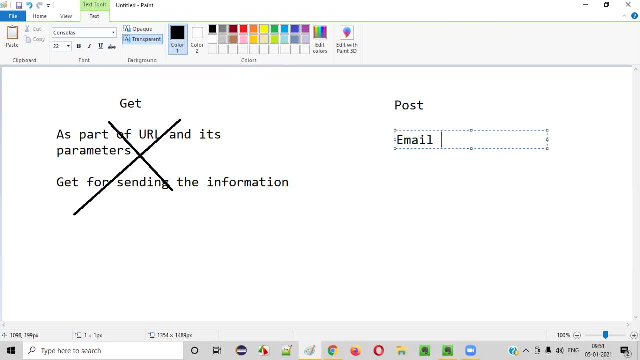 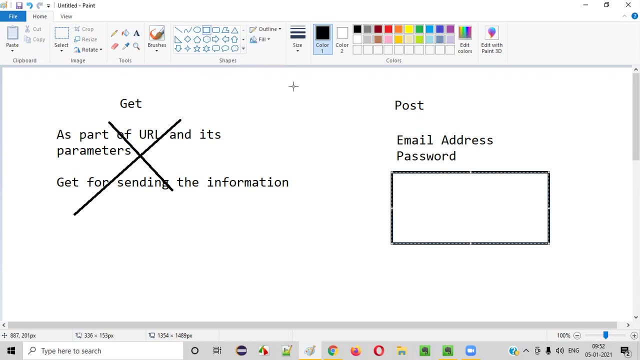 when you, when you send some sensitive information like email address and password via this post http method, then post will not use this email address or show this email address or password in the url. rather, that will be sent as part of the body- guys, body or headers, you can body kind of thing, okay. 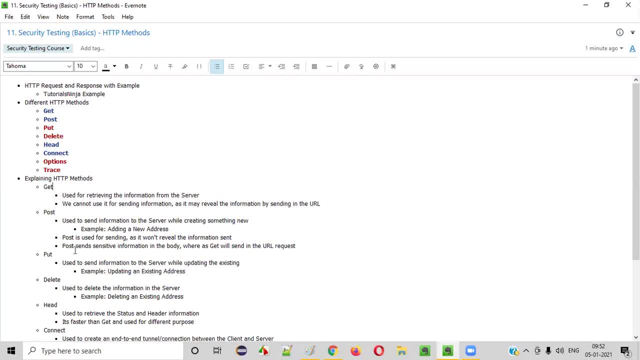 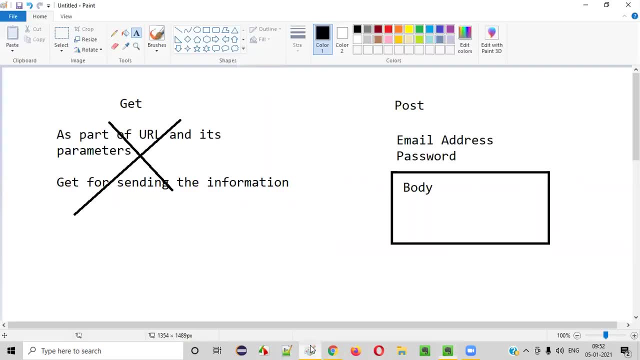 the body or header, the information will be sent. so let me show you where exactly. yeah, post sends sensitive information in the body, whereas get will send in the url. so when this particular email address and password is sent in the body, that will be in some kind of encrypted format, guys okay, that no one can read during that process of. 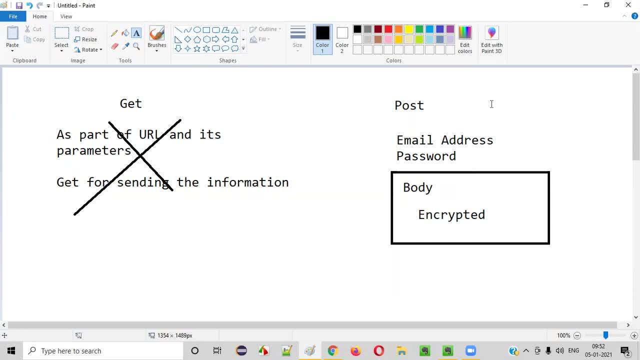 reaching the server. this information cannot be read from the body by the hackers or some other people who are interested in finding out your stuff. fine, so that's why post is secured when compared to get post is secured, guys. that's why post is secured when compared to get post is secured. 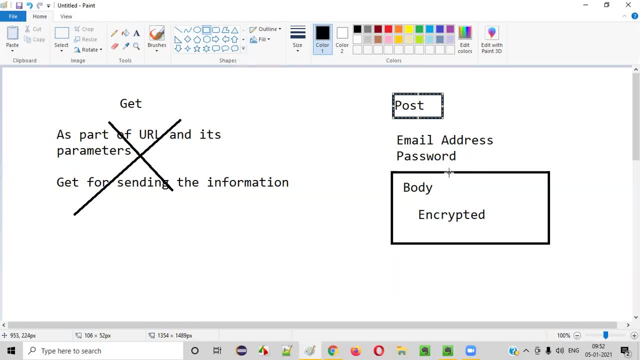 guys where your sensitive information or any information that you are sending to the server will be centered in some kind of format: uh which cannot, which is not actually openly relieved, uh which is not openly available in your url, or something. okay, so in case of get whatever the credentials you are sending, that can be visible in the url, whatever. 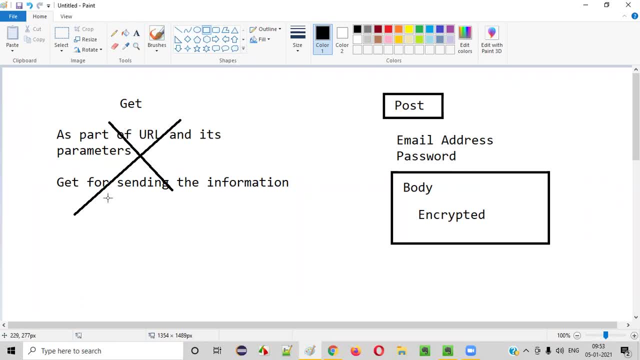 the data or credentials you send. that can be visible in the url if you use it for sending purpose, but that's why we should not be using, in case of course, for sending purpose. for sending the information to server, we'll use a post. but uh, whatever that information or details sensitive. 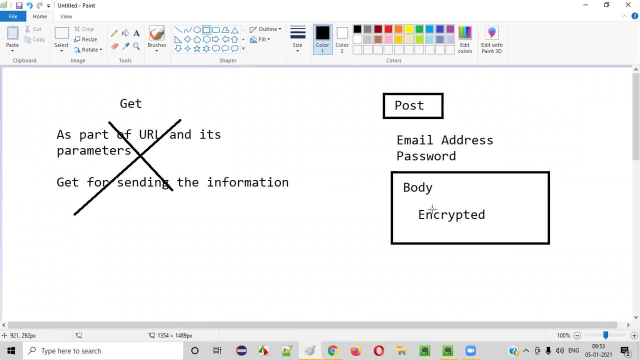 information or normal information, whatever it is. that information will be sent as part of the body section of the post. okay, you'll understand more about body and all in the coming sections, guys, so for now, just understand this. email address and password or any other sensitive information will not be sent in the url in terms of post. that's why it's secured and use it for sending. 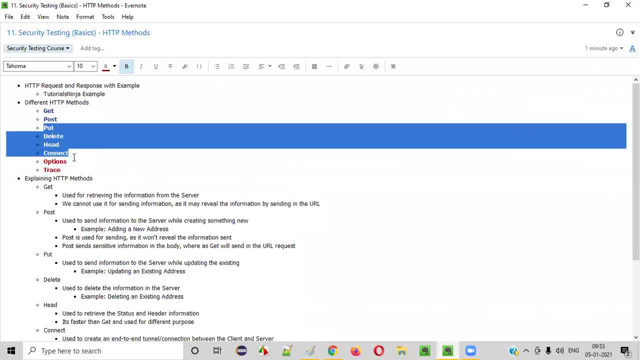 the information. so what about the other methods, guys? uh, we'll. we'll cover the other methods at a high level, guys, you don't have to dig this much deep, like data and post. so other methods. coming to the put method, put method is similar to post. okay, put is also for sending the information. 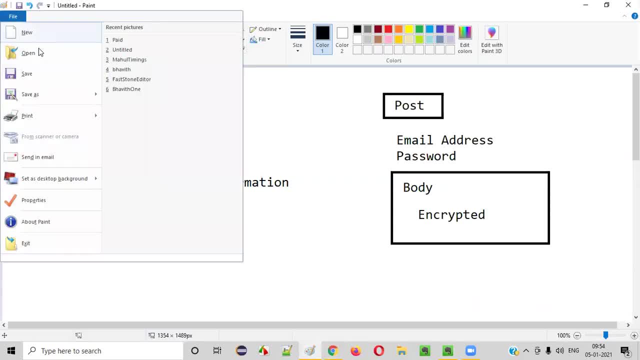 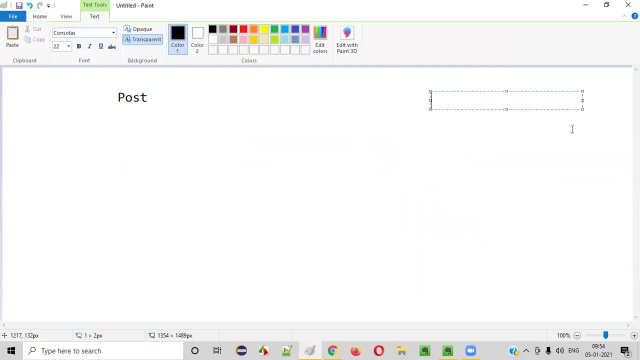 okay, so here the simple difference between put and post. i will explain so that you can understand. so we have post method and put method. what is the purpose of post? http method, i already told you for sending the, sending the information to the server from the. you are sending the information to the server, right? this is the post purpose. coming to the, 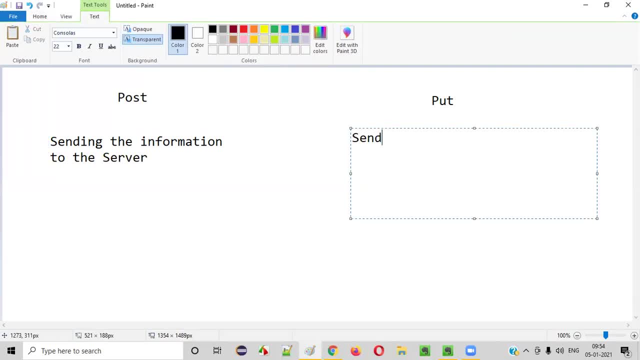 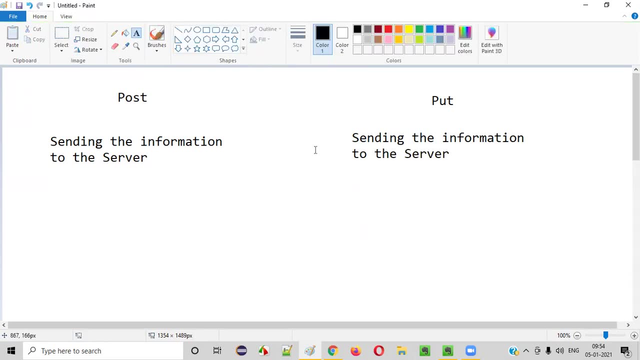 put. coming to the put here also, you are sending the information to the server. but what is the difference between the post and put? both the things are same, right, but the difference is post is generally used while creating new content, so if you are sending the information with an, 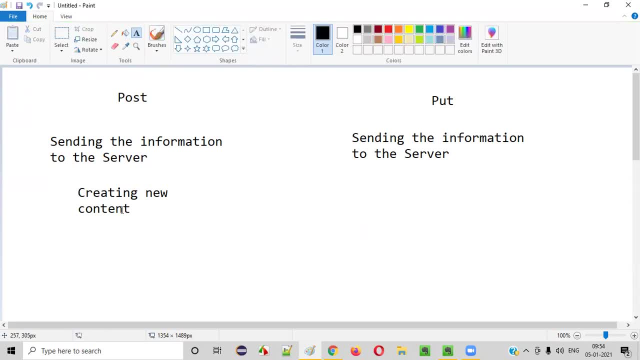 intention of creating some new account in the application or some new address. creating some new account in the application, then post is used, guys, but where put is used for updating the existing records, updating the existing. let's say you are updating the existing address. okay, some address is already added by the post. now you are. you want to edit that? you want to? 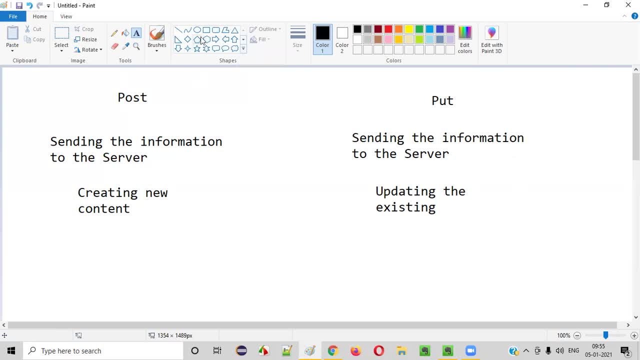 update your address for updating purpose. put is generally used, guys. okay, post is used for uh creating. if you are creating some new content, for example, if you are creating some new address in the application that i have shown you just now, then post has to be used. if you have to update the existing address, you have to edit the existing. 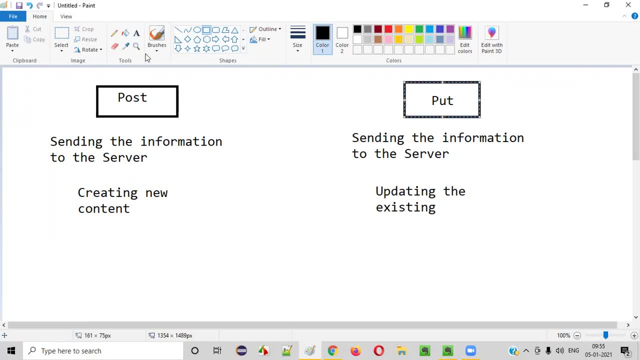 address then put has to be used. so hope you got the difference. and similarly, there is one more method, guys: delete method. as the name speaks, delete method is for deleting the existing information. if you, if you, if you want to do something where you want to delete the existing, 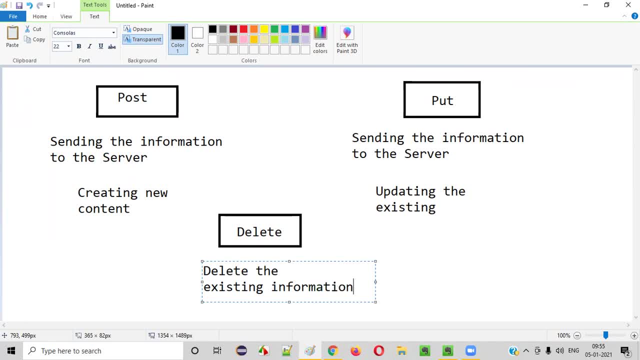 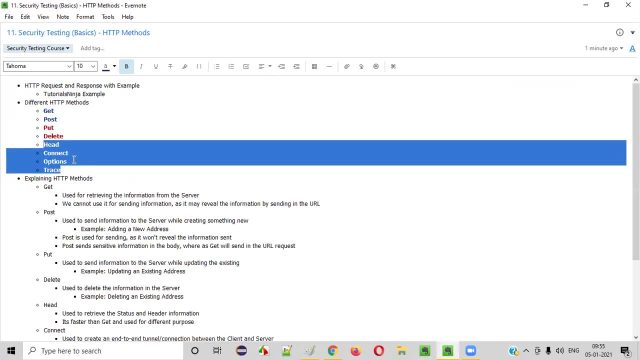 information- okay, existing information from the server- then we generally use delete. so these are the post put and delete. now we have some other. these are general, mostly used uh http methods. are these first four guys: okay, get post, uh put and delete, or the. we generally call that as crud guys: okay, crud means uh crud. 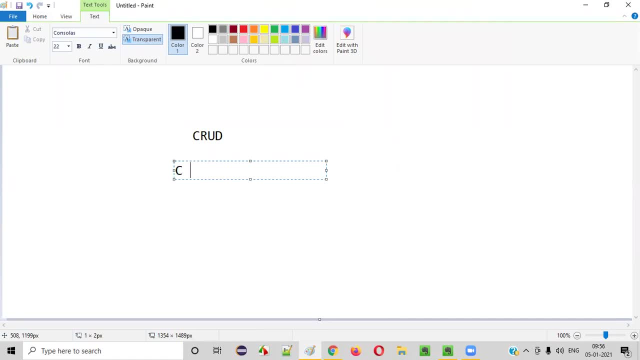 so crud. c stands for creation. okay, c stands for creation, r stands for reading, u stands for updation. in the crud word, u stands for updation and d stands for deletion. so can you categorize uh, this, uh, whatever the http methods i explained so far, into this crud? 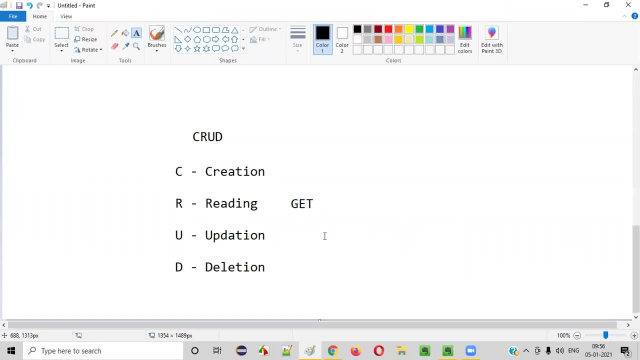 so for uh reading, we use get right for getting the information. get for uh creation, newly creating something, what you are going to use post for updating the existing records, you have to use put http method, and for deleting the existing records, we have to use delete http method. so 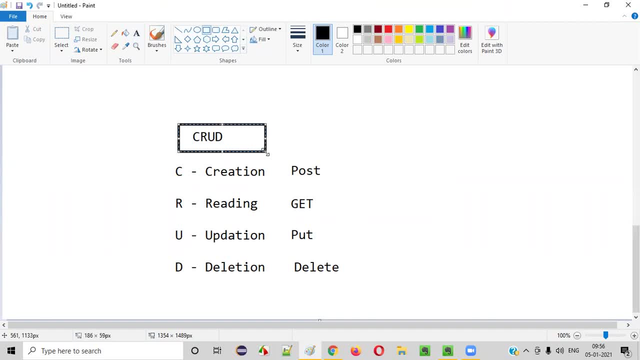 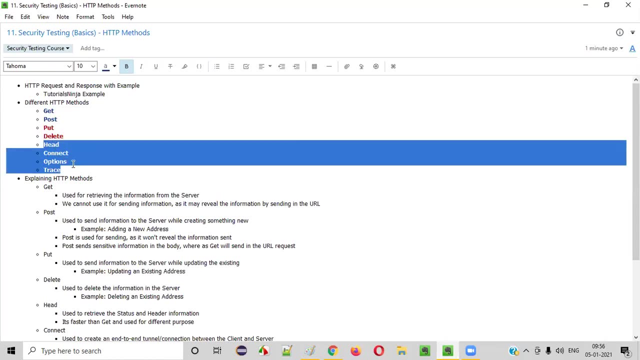 this falls in the crud and these are the basic and general. okay, generally used uh http method compared to the other http methods. we also have a few more http methods, guys, which are used for some advanced purposes. fine, so coming to the head, connect options and trace. i'll explain what is head. 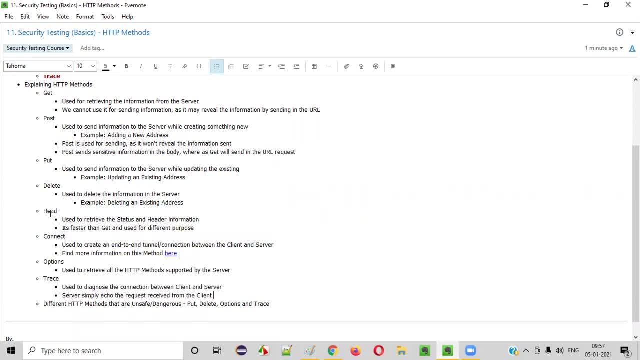 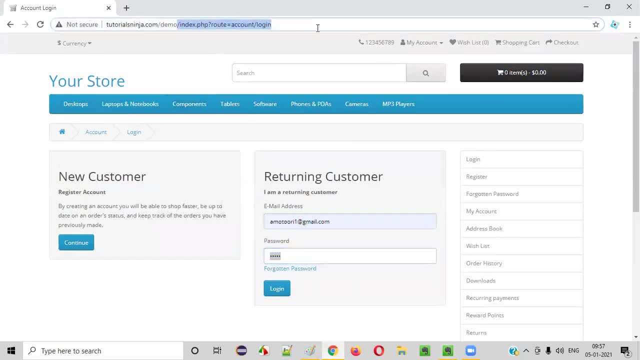 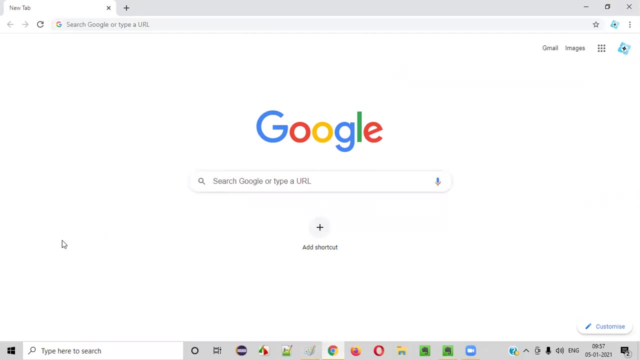 and at high level, explain head connect options and trace guys. so coming to the head guys user to retrieve the status and header information. so what does it mean? so, for example, i'll go to the basics again, so i'll remove this url also and i'll start freshly. inspect the inspect the things. so if i use 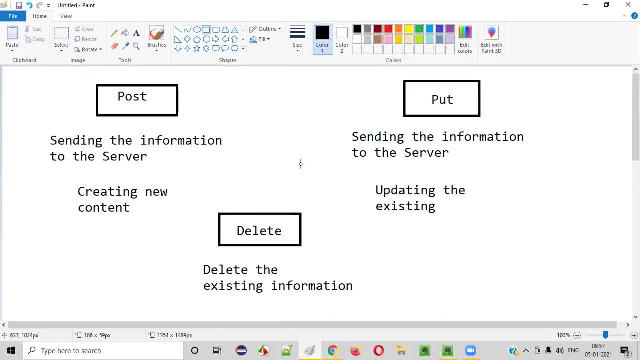 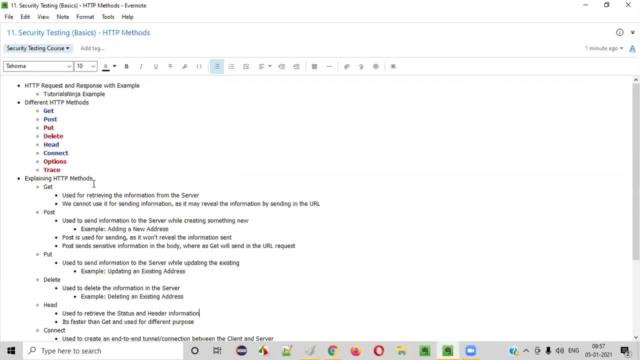 get case. there is a difference between get time. there is a difference between: so if you have to understand that head- uh, i mean sorry, what is that? so if, if you have to understand this head, you need to understand gate guys? okay, so these two need to be compared to understand the. 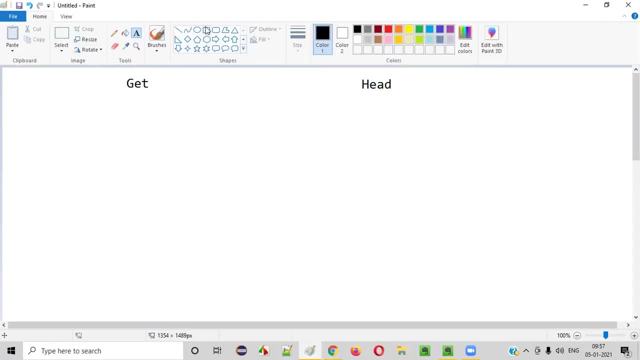 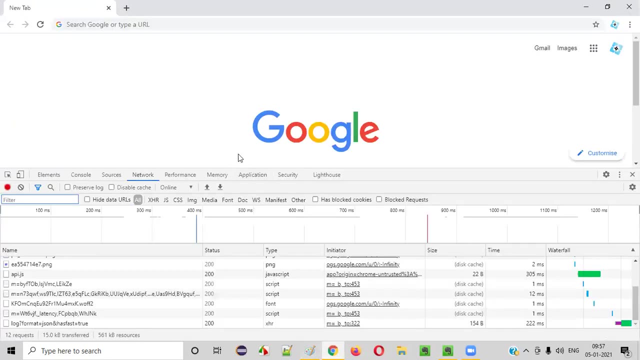 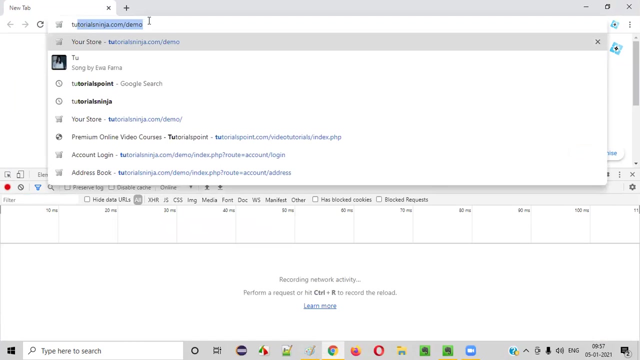 head. so fine, get head. okay, there are two http methods: get and head. if you understand the difference between get and head, you will understand head properly. fine, so first i will show you what is the difference between get and head. so here i'll clear it out and open the i'll. i will just 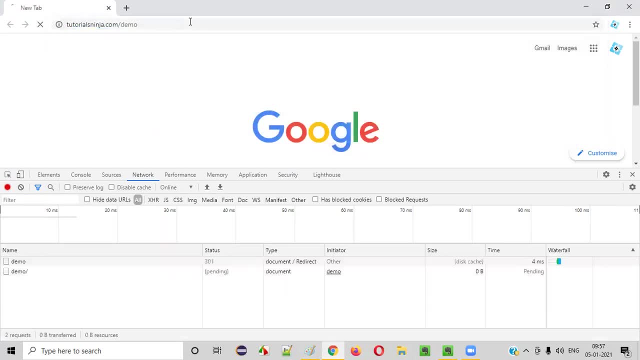 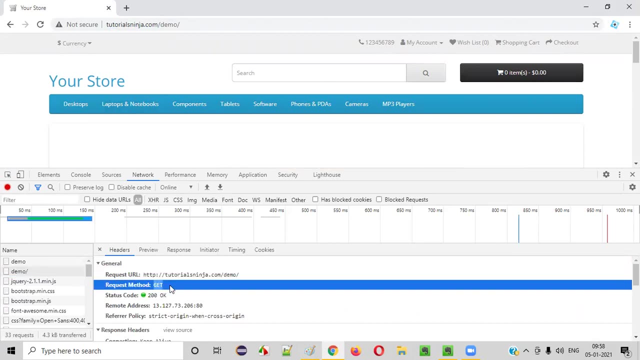 submit this url so that this request will be sent to. the get request will be sent to the server right. click on this. when i hit this, you see a get request has been sent to the server right? this is a url and this is the get http method request. fine, so you'll get some response also, guys here. 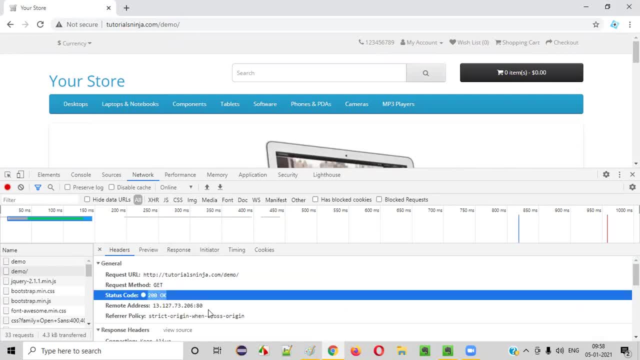 right, you are getting some response and also you are getting some status code. status code is coming, response is coming and also response headers are also coming. right, so what exactly you are coming from the server? so in the request these two things are sent in the request case: request url and http method. 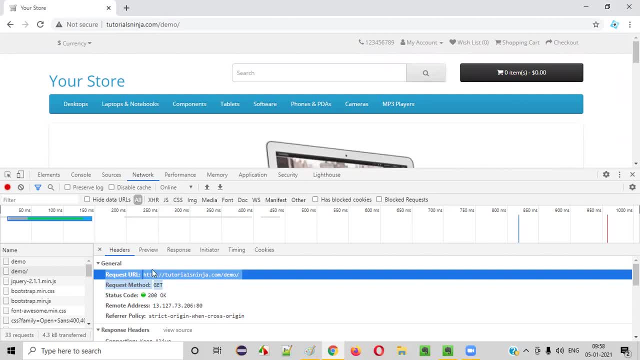 that is, get will be sent in the request to the server. from the client to the server. these two things are sent as a response. we got this html code in the response and along with that html code we also got the status code in the response is: everything is okay, 200 okay will come okay. 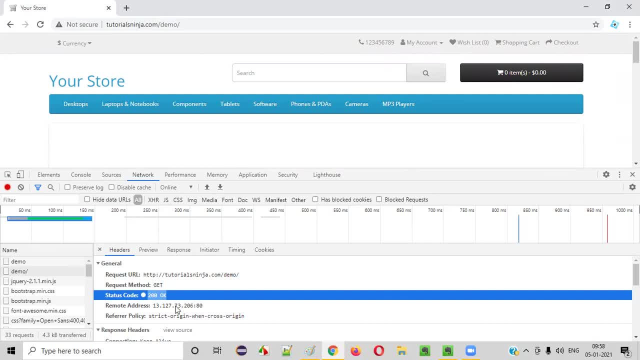 status of the request, whether it is properly processed by the application server or not. that 100. okay, along with this uh res, uh status code, we also got along with this response code and status code. we also will get this response headers. okay, all these response headers also will come. 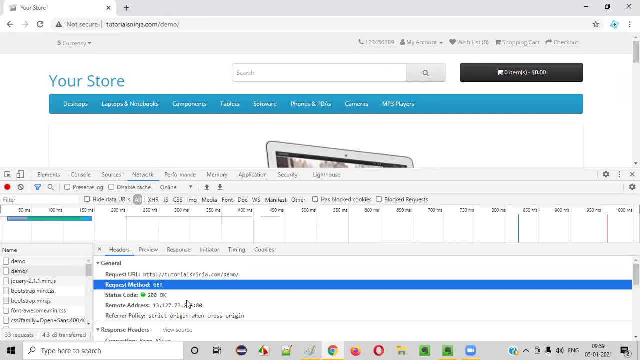 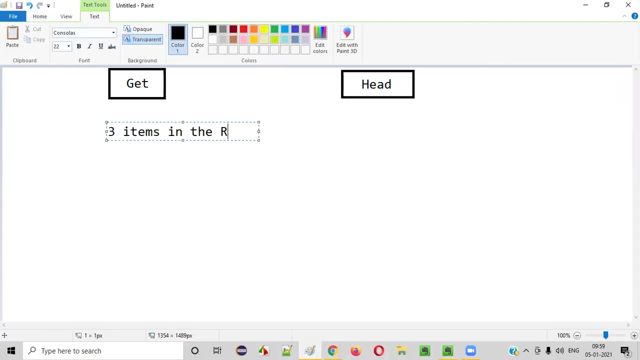 from the server. so this is what happens in the general. okay, three items. you got the response, status code, the response, html code and response headers. but, guys, here, how many items? we got three items in the response. the response. we got three items in the response. when you process the request, when the application server crosses the request. 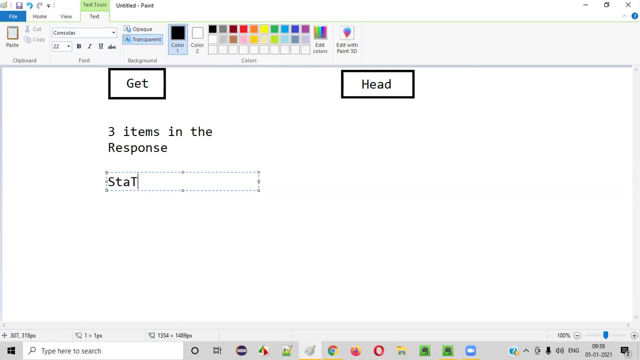 it will send three items. one is a status code, whether request is okay or not- status code, that is, status 200, okay. and other one is like a response, that is, response html code. some html code came in the response which we are using for displaying the page right. and the third one was: 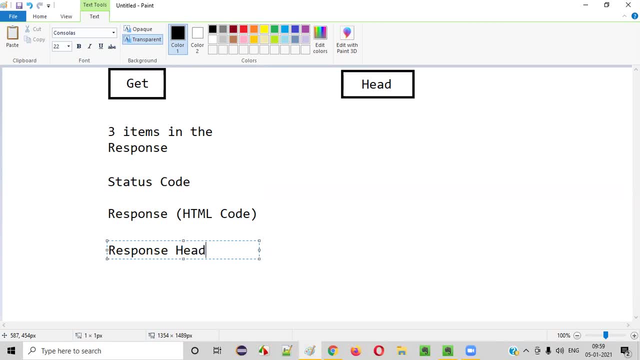 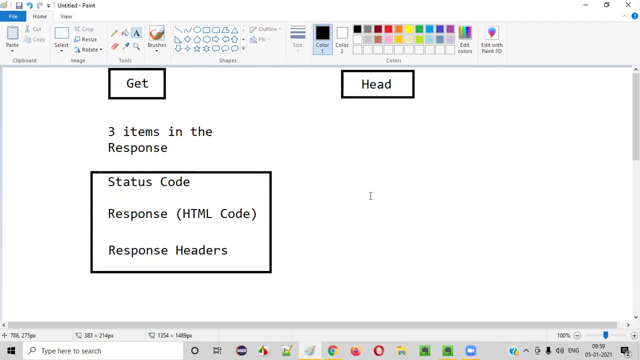 response headers. but in case of head, guys, you will not get all these three items. okay, in case of hand, you will only get two items, that is, status code, whether the request has been processed properly or not, and uh, response headers only. okay, i don't have an example to show you practically, guys, but uh, this is what uh will happen when you use head. 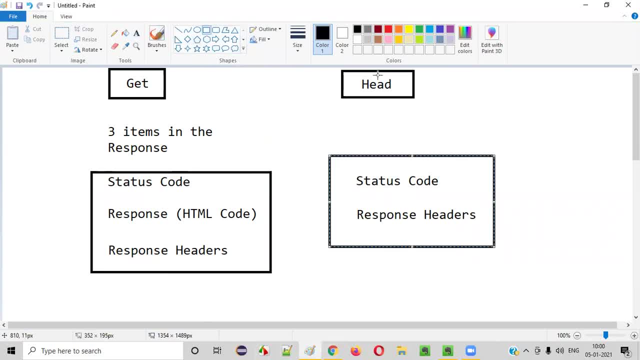 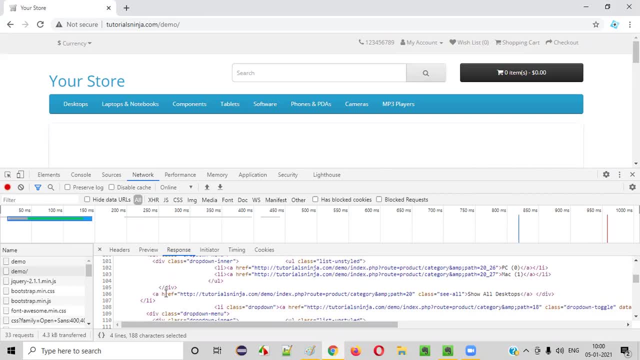 over gate. so here you will not get uh, in case of, in case of head, you will not get this uh response body, this, this is called as response body. guys. this response body will not be coming in the terms of head. this response body is coming because the 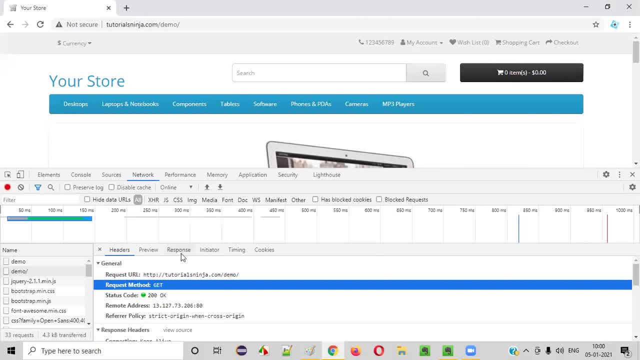 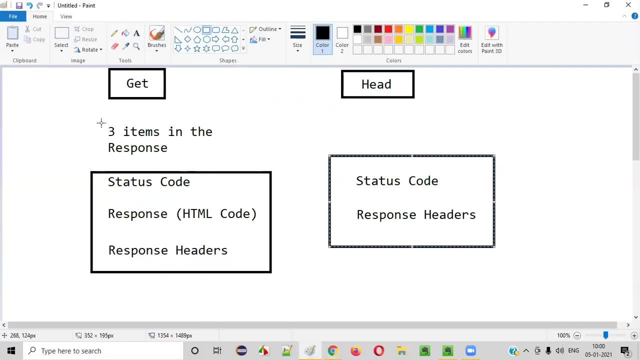 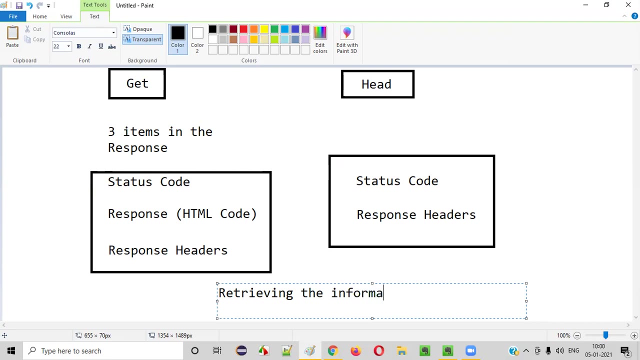 used is get guys in case of head. if this method is head, in that case nothing will be displayed in the response body. fine, okay, so that is the difference between get and head. both are same. both both are used for retrieving the information from the server. these are for from server. from the server you are getting the information head and 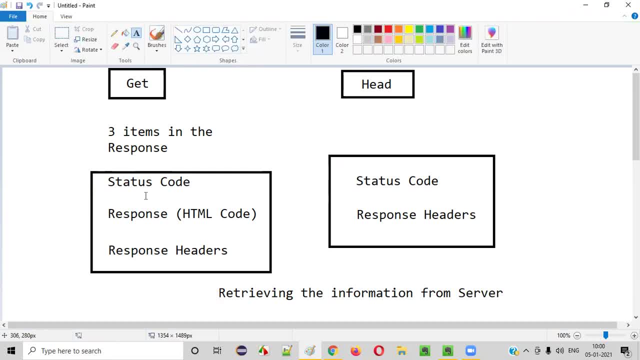 get and head are used for retrieving the information from the server. where get will get you all the three items like status code, response and response headers, where head will only get you the response code and response headers only. okay, so the html code kind of response, uh, uh, response body, such kind of things will not come guys. okay, you'll not get that kind of things. 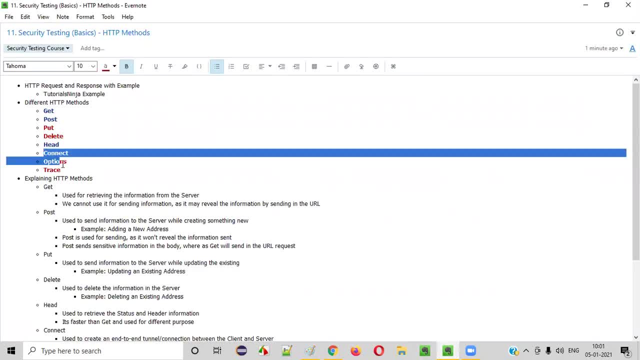 from the head when you use head. so hope you understood what is head. now the other three things, that is, http methods, that is, connect options, trace. at the end of this session, guys, i'm going to explain you what are the. i'm going to explain what are the safe methods and what are the dangerous methods in terms of security, guys. 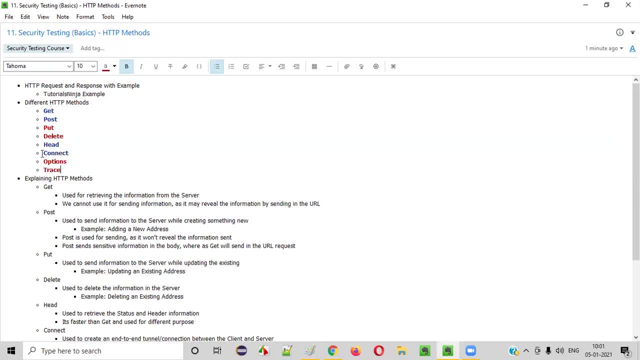 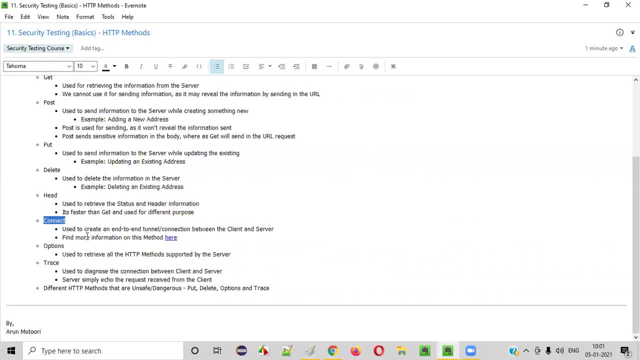 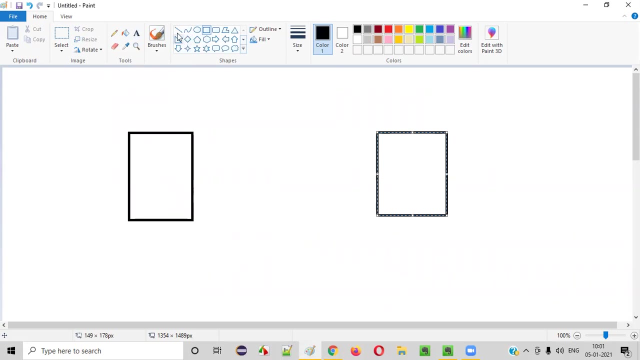 just be tuned till we complete the remaining http methods. so the next one is connect guys. what is the purpose of the connect? so connect is used to create an end-to-end tunnel connection between the client and server guys. so let's say this is a client and this is a server. okay, so a end-to-end. 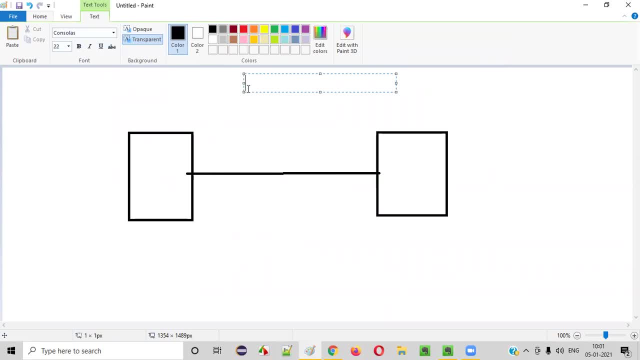 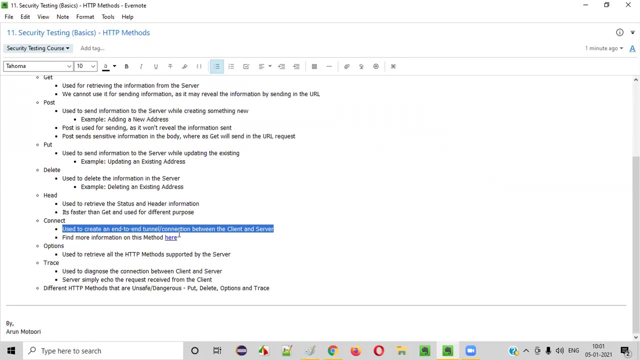 tunnel will be created. a communication channel will be created using connect, so you don't have to dig it to depth. okay, so end-to-end communication will be created with help of this connect. okay user to create an end-to-end tunnel connection between the client and server. 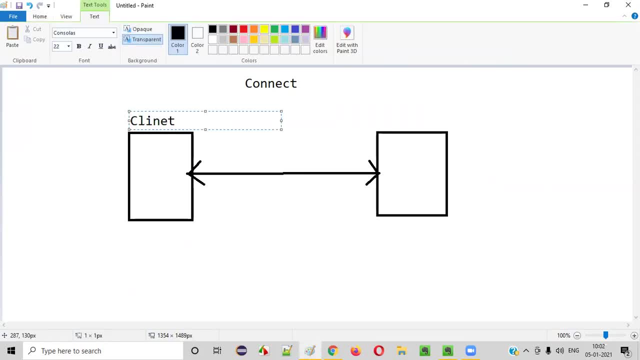 this is a client. let's say this is a client where you have opened your application in the browser. that's the client and this is the server application server. so a connection has been. if you want to establish a connection between this client and server, then you'll use connect. 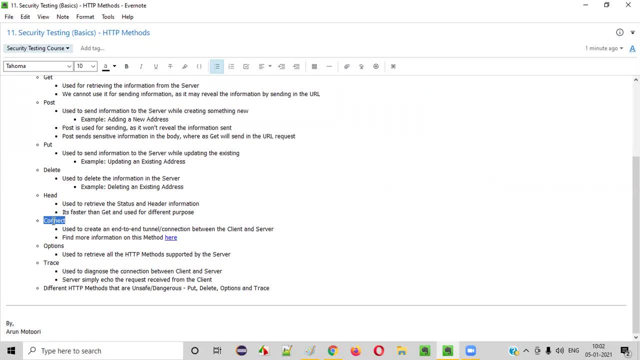 so so it's very technical guys. so, uh, we have to go out and of the topic if i have to explain what exactly the connect is all about. so, if you really want to explore what is, what exactly is the main purpose of the connect, uh, here in the notes, guys, i'll be. 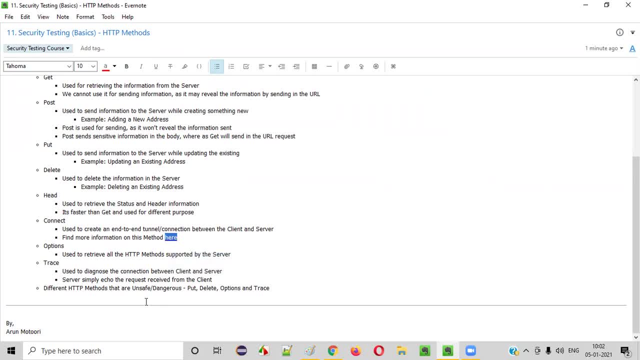 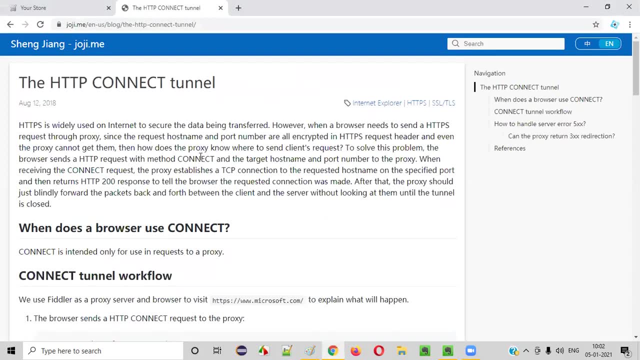 providing these notes in the along with the video, so you can go to this notes and then this notes and then you can access this url, copy this url and open it here, this particular page. okay. so jojime enus, block the http connect tunnel. okay, if you browse this url right, you'll get all. 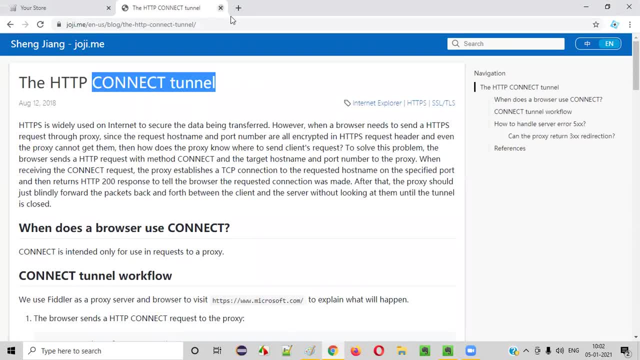 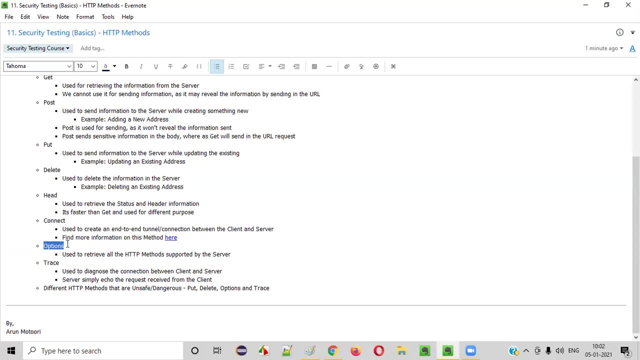 the information about what exactly is connected to that url. so we're going to proceed with the. this connect http method is all about. so it has a lot of thing, so i don't have to cover in this session because it will deviate my session. fine, next one is options. so the next one is options. 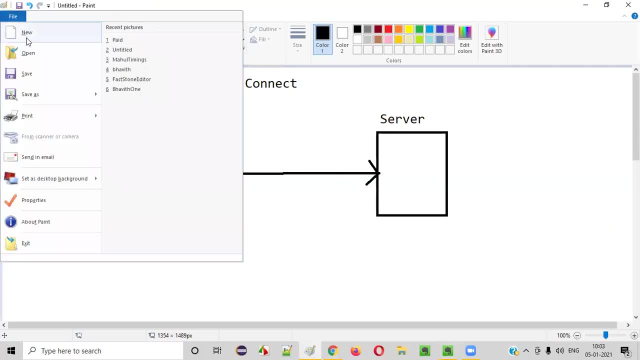 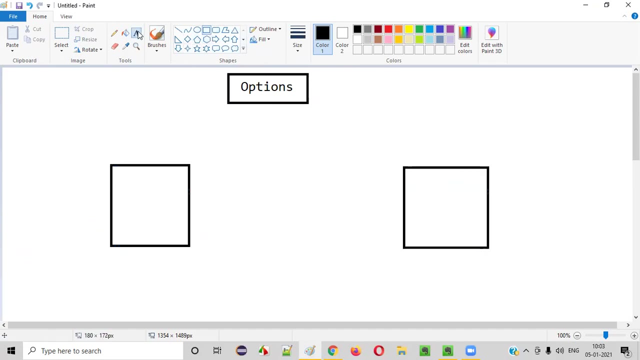 so what is the purpose of the options? we are done with the connect and let's next http method is options. so what is the purpose of these options? if you want to know, okay, if you want to know, let's say this is a client and this is a server. i'll write it here: client and server. 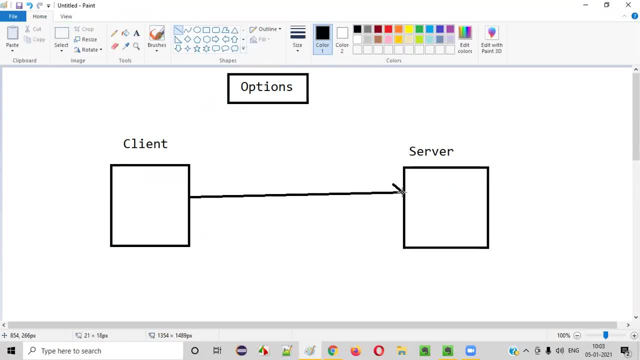 if a request has been, a request has been sent from the client to the server with this particular options. okay, with this options, http method used, what happens is this server will process this request and send in response all the. the server will send all the the response. what you'll get this: 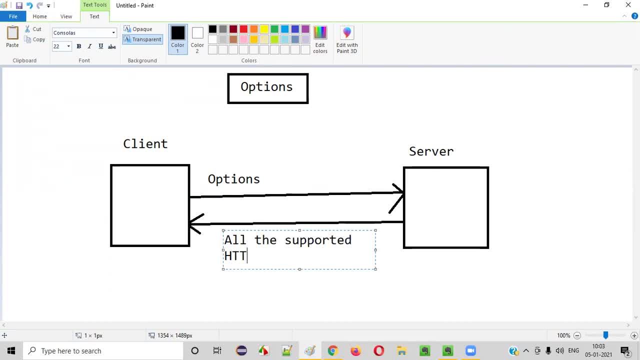 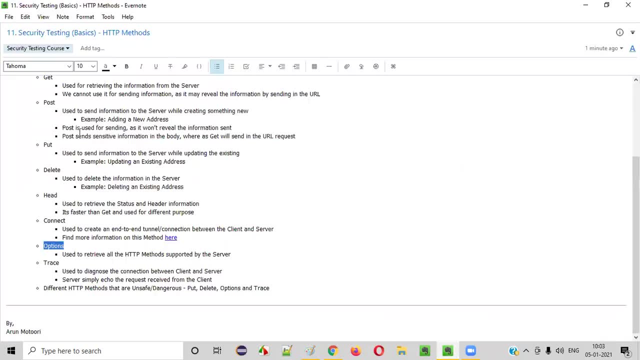 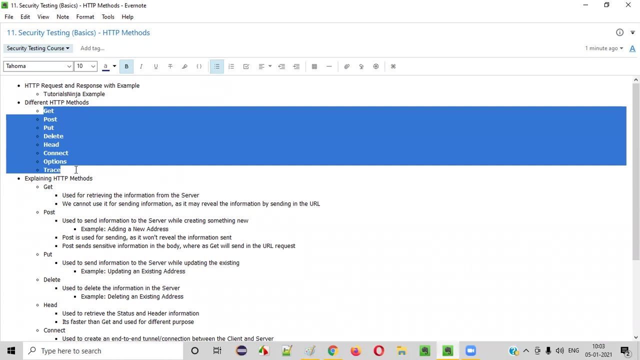 all the supported http methods. okay. so some servers, guys, some some server will not support some http methods. so it's not compulsory that all the history methods need to be supported by a application server, some server, some servers- what they do is some application server, they will disable some http methods. okay, they'll. they'll only allow you to use get post kind of thing. okay. 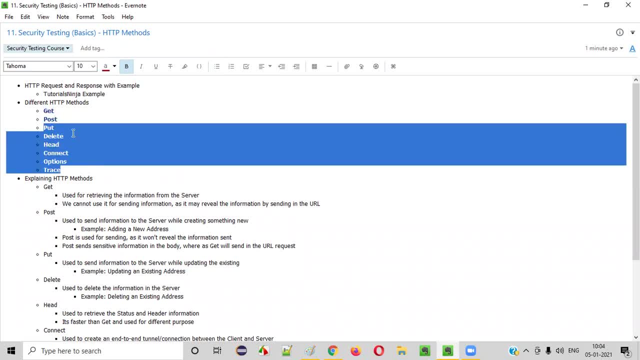 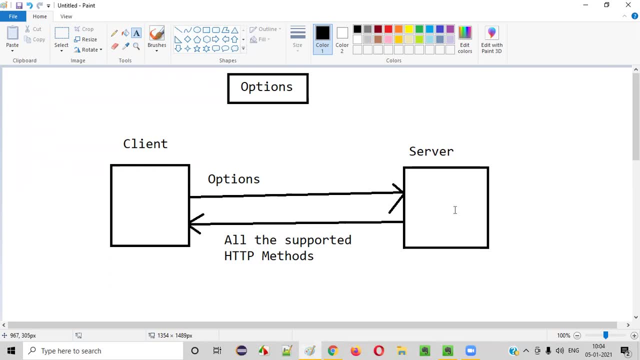 they'll not use. they'll not allow you to uh use this other http methods. so what are all the supported? what are all the supported http methods by this server? if you want to find out, then we have to use options http method when you trigger this request having the options. 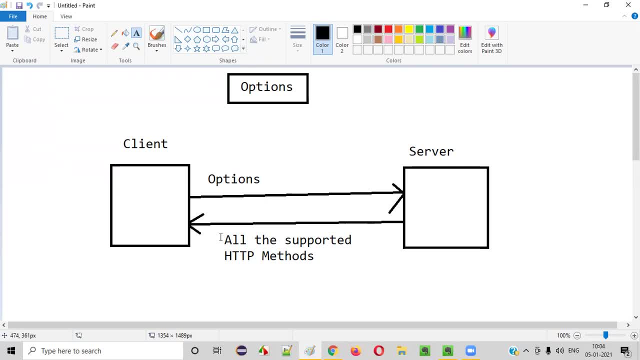 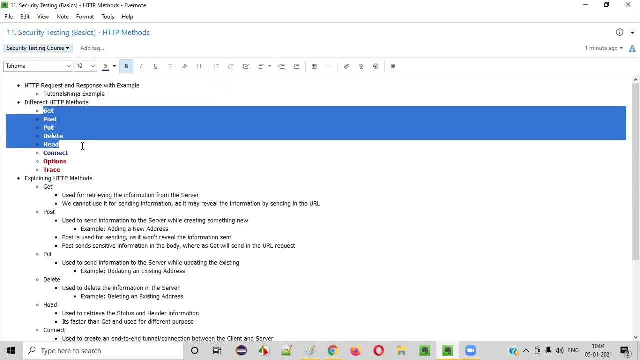 http method, then server will process that and, as a response, it will let you know what are all the methods that are supported by this server. okay, if the server is supporting these five http methods, then it will list all these http methods that are supported by the server. okay, application server. fine, that's what. 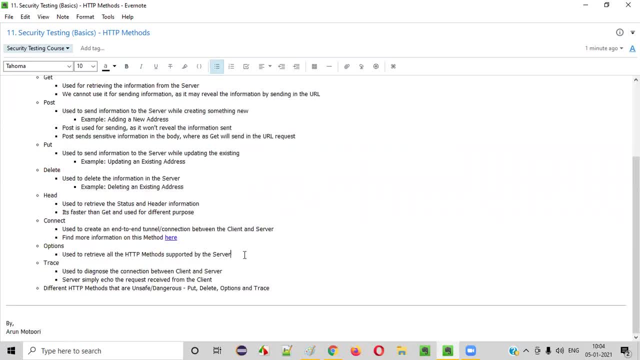 is the intention of this options guys. and next one is trace case. last one is trace. so what is the purpose of the trace? use it to diagnose the connection between the client and server, whether the connection between this client and server is proper or not. if you want to diagnose, okay, if you. 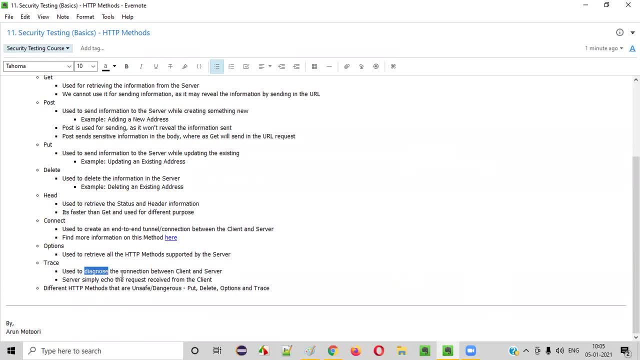 want to run a diagnostic kind of check to check whether the the connection between the establishment between the client and server is good or not, then you have to use trace, so it will simply echo guys. okay, whatever the request you are sending the, the request details will be echoed back. 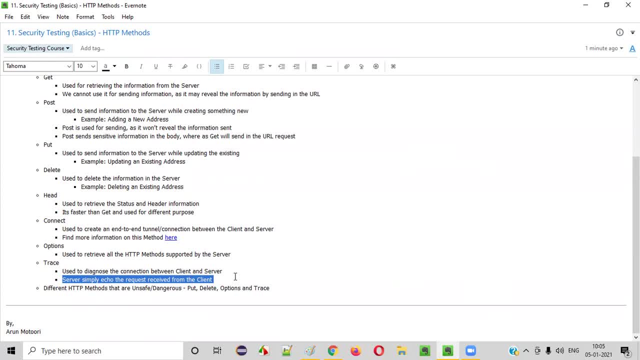 okay from the server, just to confirm that the connection is good. okay, so generally this kind of trace, kind of http method will be used by the developers for debugging purpose. okay, so this is generally used by the developers for debugging purpose. guys, we don't have to dig that much deep. 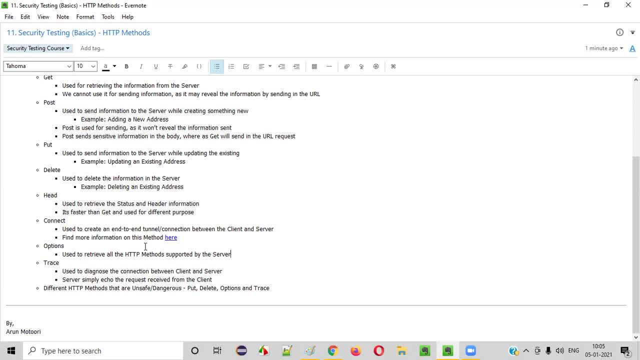 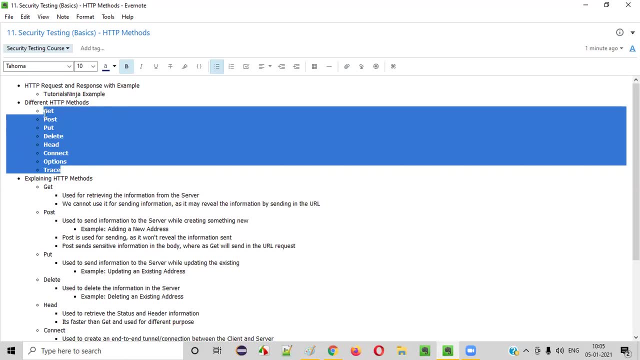 fine. so that's fine, guys. now the term has come. the term has come to find out which out of all these http methods are safe to use and which out of all these http methods are unsafe or dangerous to use in terms of security testing. okay, so coming to that. 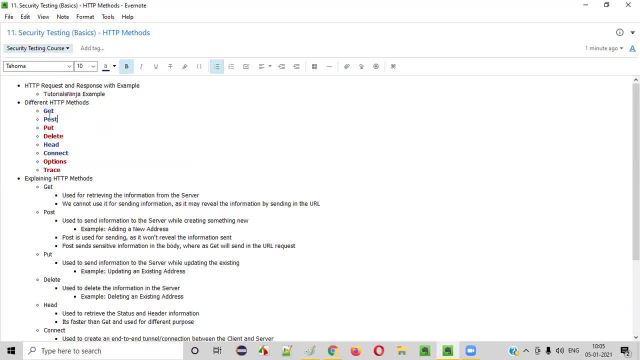 so here, as you can see, the color guys, okay, i have, i have written some. i have just mentioned few http methods in blue color and few other http methods in red color. the red ones are dangerous guys in terms of security and the blue ones are safe. okay, get and post are safe, head and connector safe. 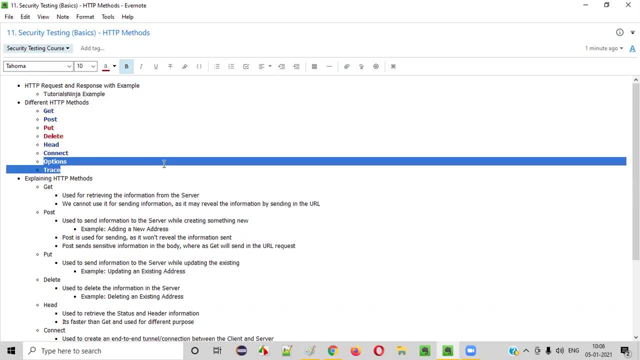 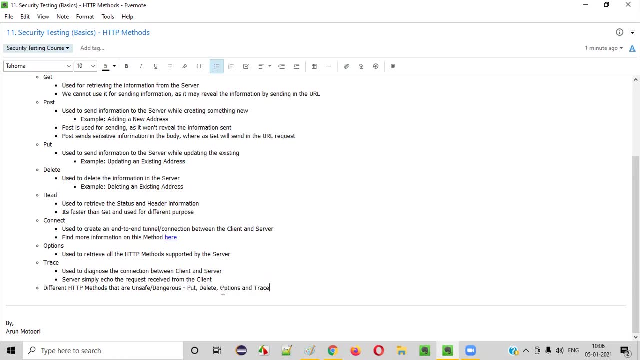 whereas put delete options and trace are not safe. they are dangerous guys in terms of security. put delete options and trace http methods are dangerous guys. why? because, if i take the example of delete will delete some resource, right, so in terms of that it is not safe. okay, so we're coming to the 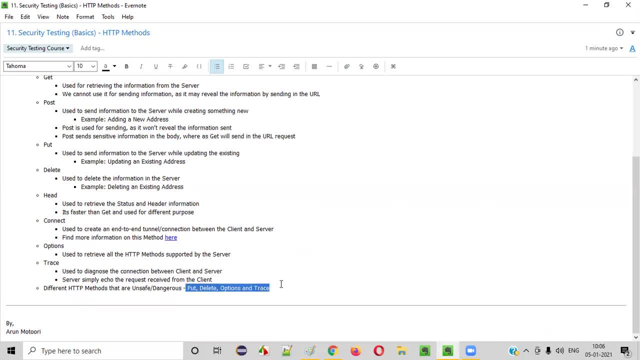 options options is also dangerous. i'll explain more about why these methods are dangerous in the upcoming sessions in detail, but for now, at a high level, understand this will modify the resources or delete the resources. that's why it is dangerous in terms of security options will let you know. 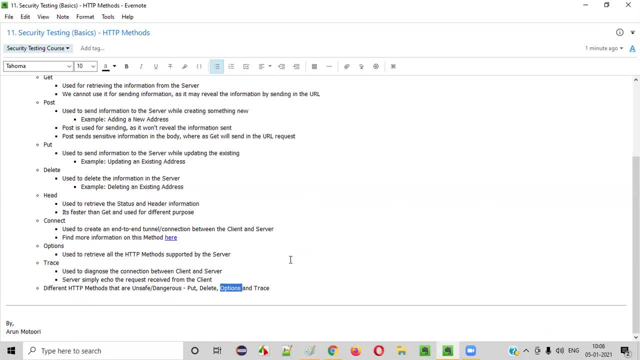 all the supported http methods. if a hacker want to find out what are all the http methods that are supported by this application, you can simply put a request to the server saying that, with options http method, then if server gives the hacker the information that these are all the. 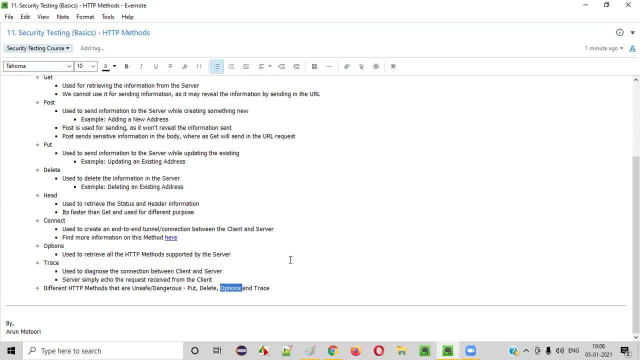 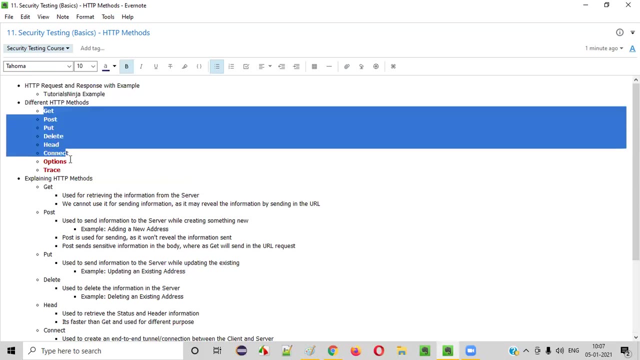 supported methods by the server, and if some of the unsafe or dangerous http methods are available, hacker can take advantage of that. somehow at some level you can. this option's extreme method is revealing some security information- right, secured information so. so an application should not reveal what are all the extreme methods that are supported by it. 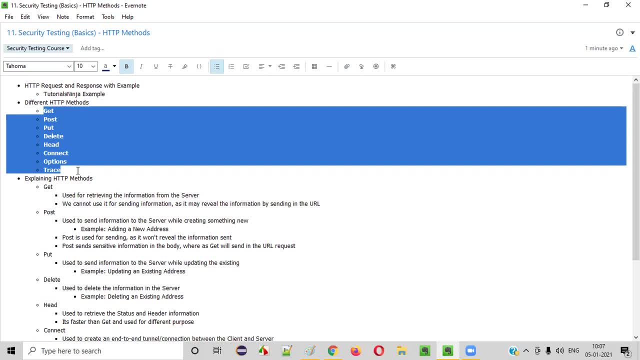 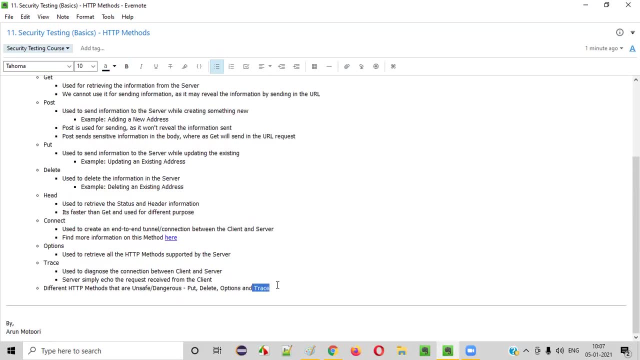 okay, that's the main problem. if the hacker find it out, it can take advantage of the http methods which are not secured. fine, so then next one is also. next one is trace. guys, uh, somehow trace is also a dangerous kind of http method in terms of security. we'll explain more. 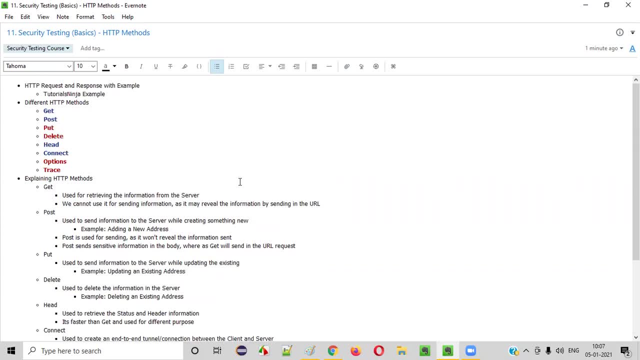 about why these things are dangerous in the upcoming sessions when the time comes. so hope, guys, uh you understood, uh the basic concepts, okay, that we started from this session for security testing and uh the topic was like http methods. hope you understood the, what exactly the http methods are.